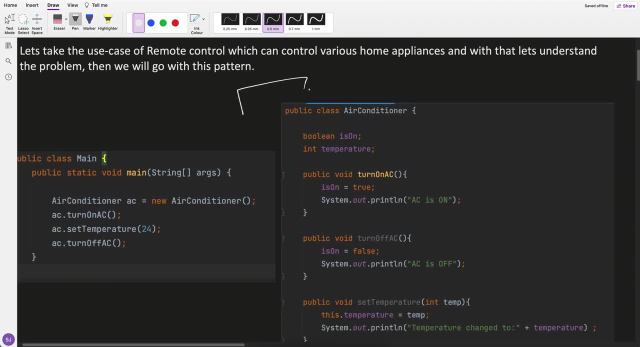 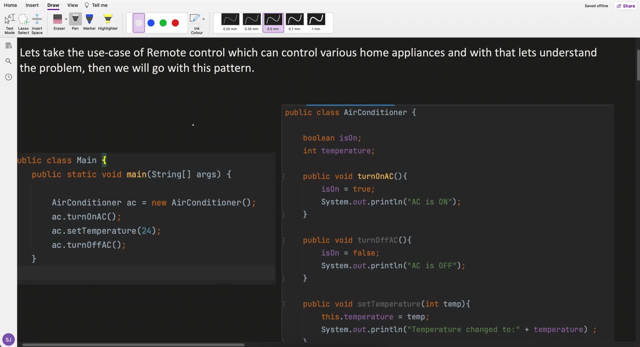 let me first tell you a simple use case and see what problem exists today, which and how command design pattern solves it Right. So let's take this example. So, as I told you, what things comes to our mind is generally remote control: text editor, cut copy command. 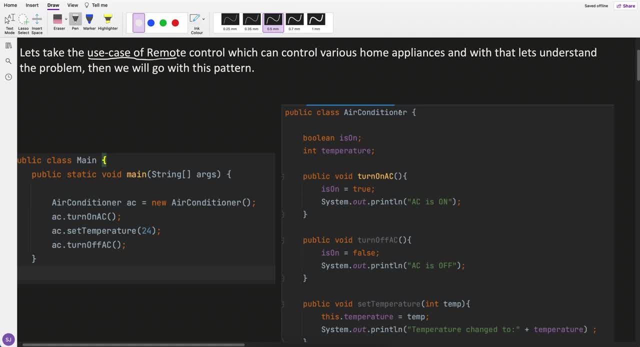 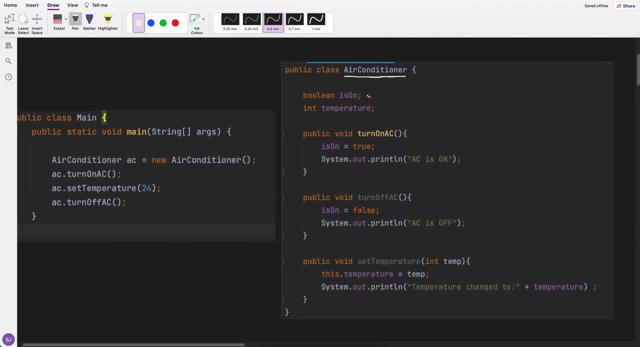 So I have taken our use case of remote control right. So I have created one simple class- air conditional class right, and what does air condition has, whether it is on or off? right. So I have created one simple class- air conditional class right, and what does air condition has, whether it is on or off. 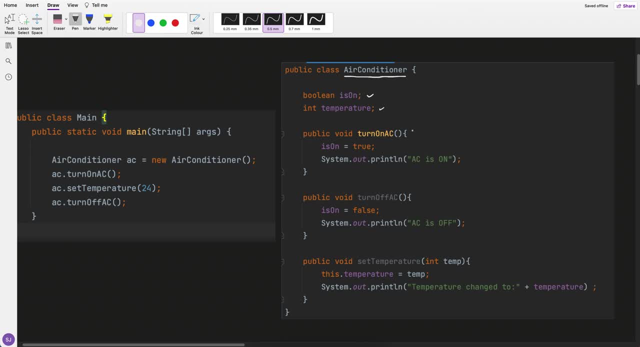 and its temperature. So I have declared one method: turn on the AC where I'm changing this flag to true and system is on. Similarly, I have turned off the AC where I'm making this flag to false and your AC will be now off state. Similarly, I have one temperature set temperature method. 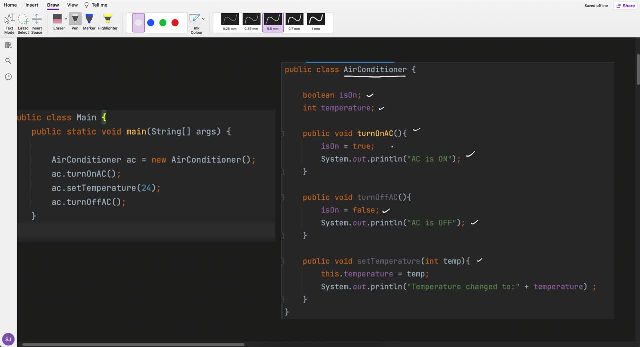 where, whatever the user wanted to decide temperature to have, it will put the temperature in the input. we will set the desired temperature. Okay, so this is very, very basic air condition class And this is your client And how client use it. 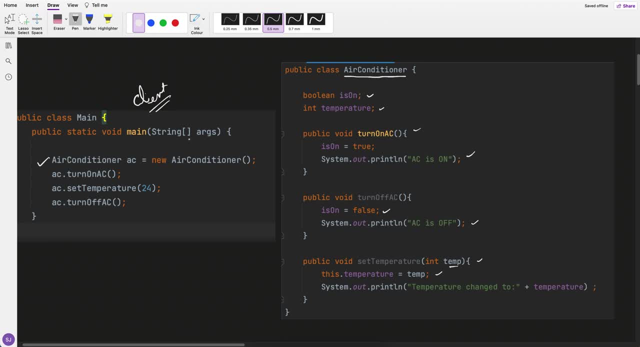 it first has to create an AC object. Yes, AC now exists. Now it will operate it. it will turn on the AC. it will set the temperature and turn off the AC. Very simple. Do you see any issues in this Right? Do you see any issue? Stop the video. 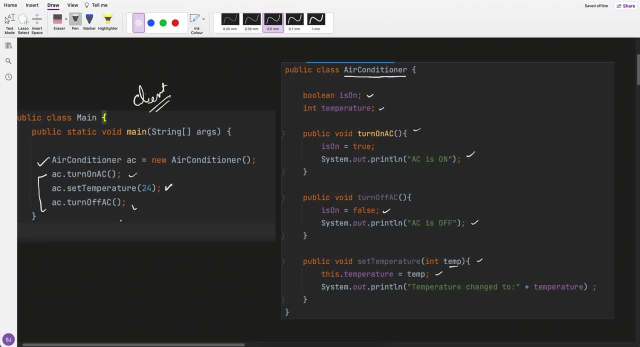 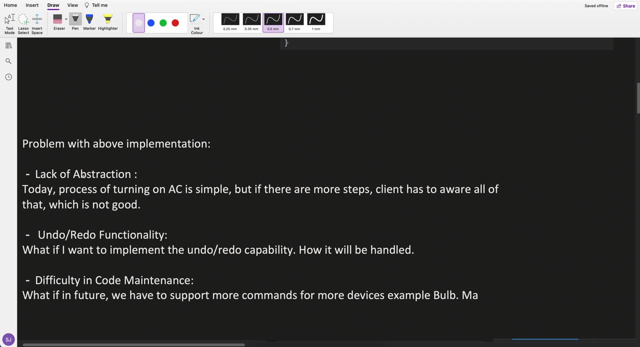 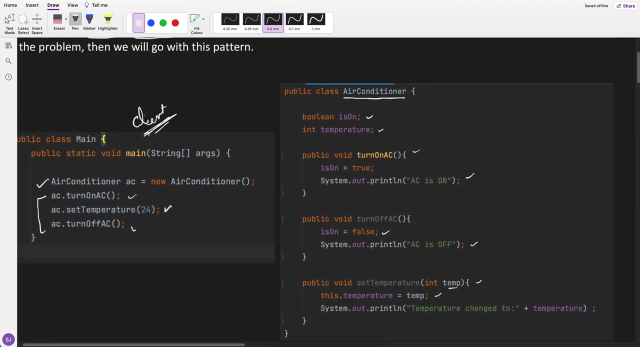 think about it, put into the comment what all issues do you think? then proceed further. So let me tell you what all the issues I see in this example. First issue which I see is your lack of abstraction. So here, if you see that the client has to have the knowledge of, okay, turn on the AC. 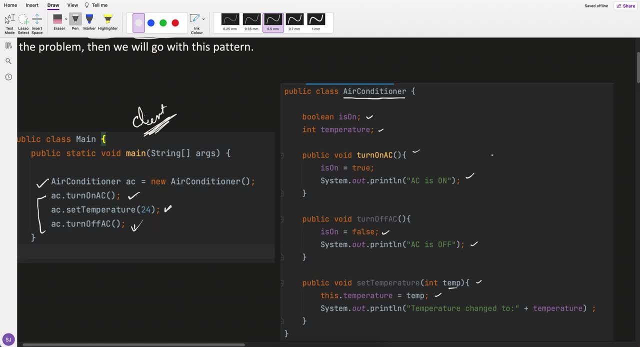 set the temperature, turn off the AC. What if tomorrow? today, it is very simple: one method: turn on the AC. AC got turned on. What if there are a set of methods is given and these set of method has to be performed to turn on the AC? Let's say that there is not. 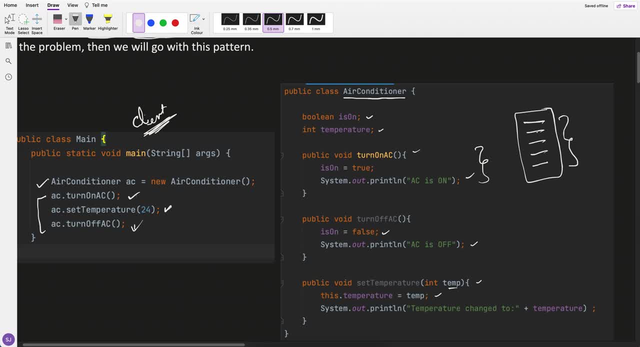 no one method exists turn on the AC. there is certain steps or set of methods exist And this method has to be executed to turn on the AC. let's say then client has to has the knowledge about that. Okay, if it want to turn on the AC, then it has to know about all these steps, Right? 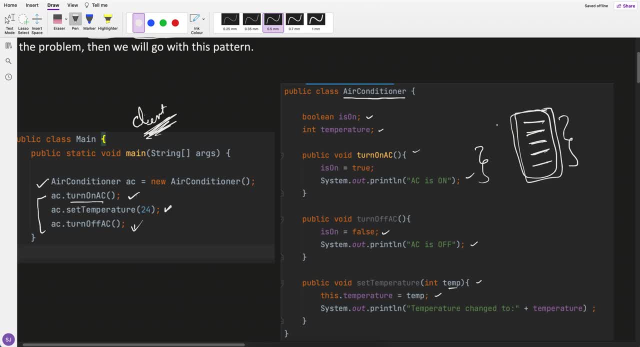 So there might be many, many internal sequence of steps might be happening when you click on the button turn on the AC. So what I'm trying to say? that let's say this is a very straightforward example. But let's say, in the real world, if air conditioned class has so many methods and there is nothing like turn on AC. 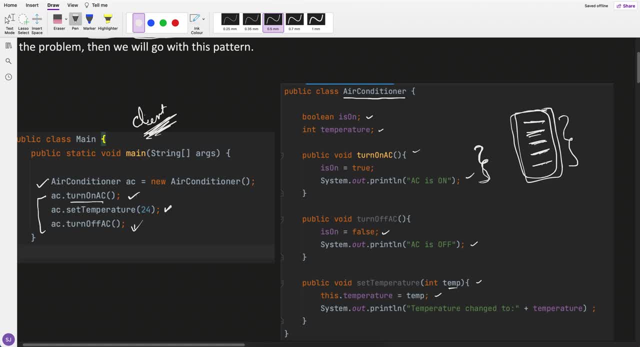 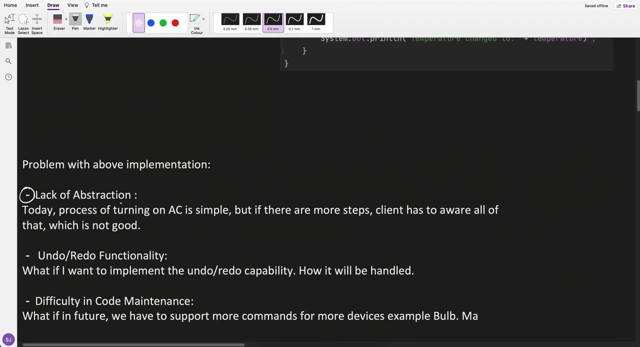 method. there might be a certain small, small methods existing and you have to perform those steps to turn on the AC. then client has to has the knowledge about or followed And any change on those steps client get impacted also. So first thing is lack of abstraction. Today process of turning on AC is 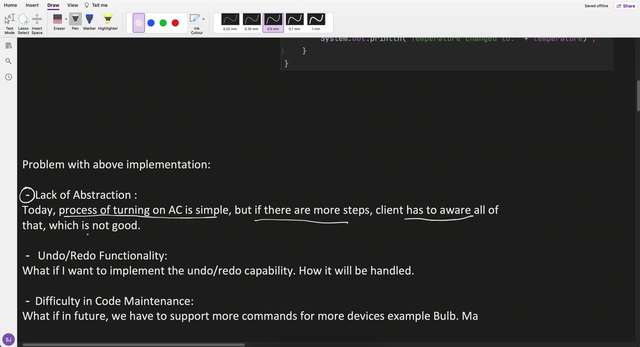 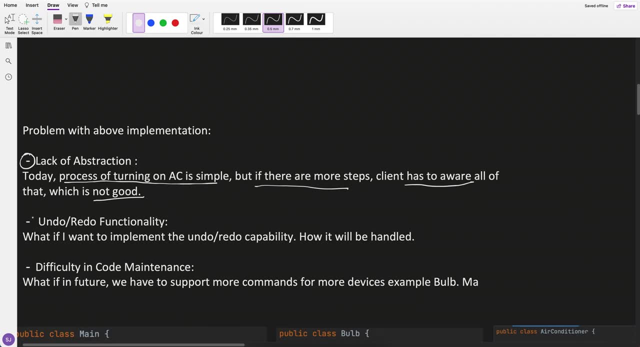 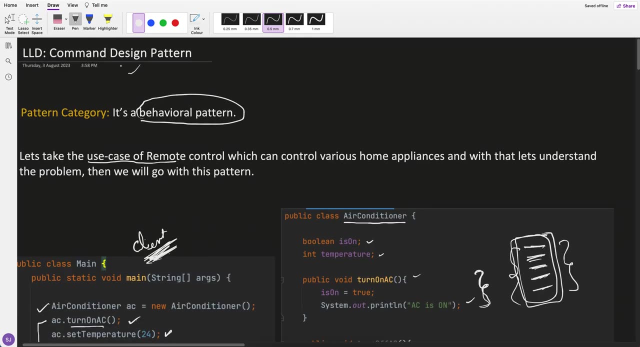 simple. But if there are more steps, client has to aware all that which is not good. So that is. first problem I see is there is a lack of abstraction. Second thing is undo redo functionality. So see whenever sometimes things is like command Ctrl C, Ctrl V, these are all command copy command. 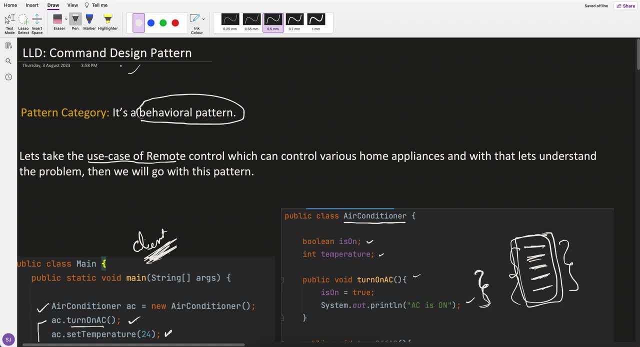 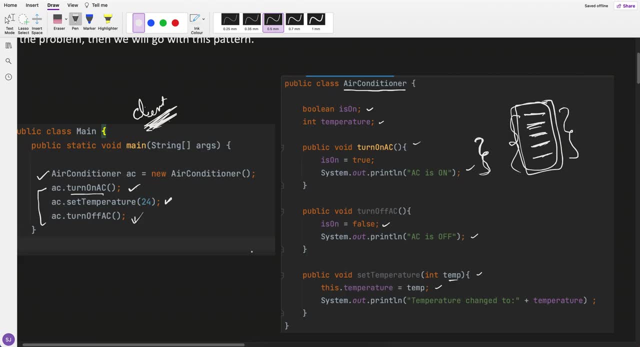 delete command, paste command. The one thing which comes to my mind is how you will undo the operation, how you will implement the undo operation, how you will implement the redo operation right. So in this, let's say, for this example, if you have turned on the AC, if you have to, 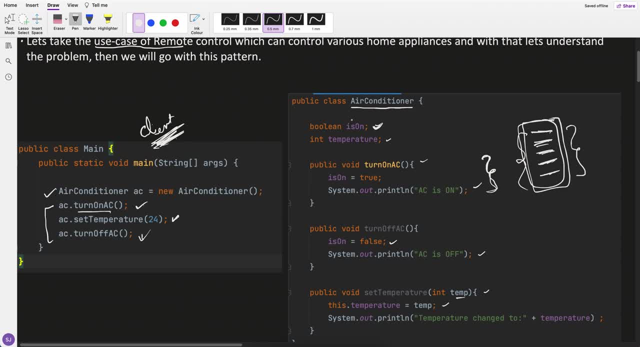 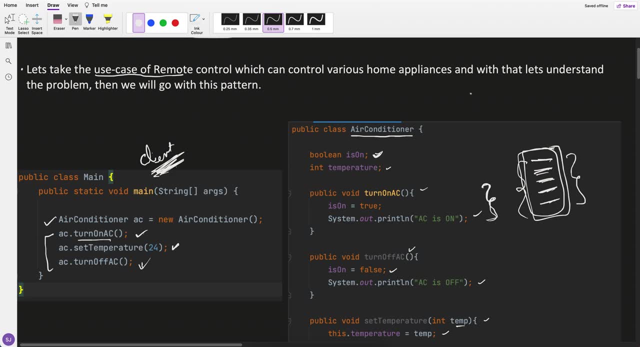 undo it right. how you will do undo it. is there a way you will? you will call another command, turn off, but that's not undoing. So let's say you have invoked 10 times certain commands Now and you have to undo it right. So that capability, how you will build it here, in the simple right, Because 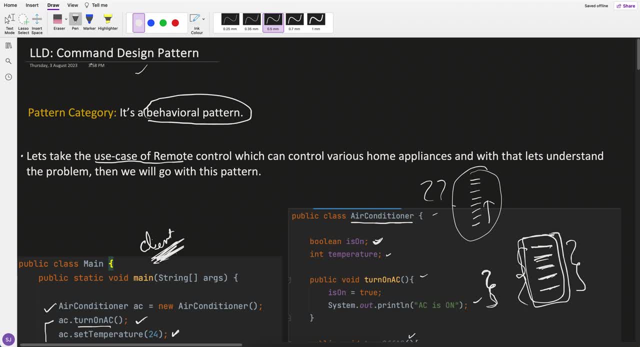 we are talking about command And you know that wherever the command happens, it's possible that we have a feature called undo. Also, this is a very, very important interview question also- how you will perform or implement the undo redo operation right, So that things which is like 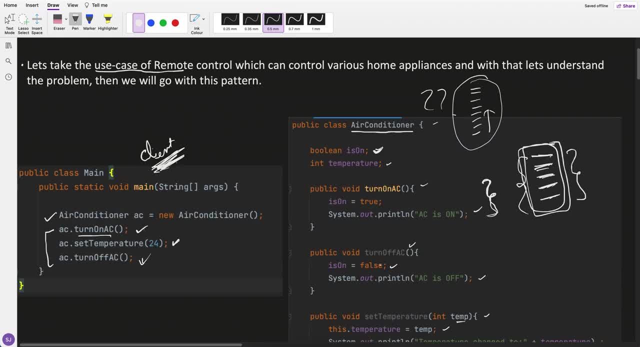 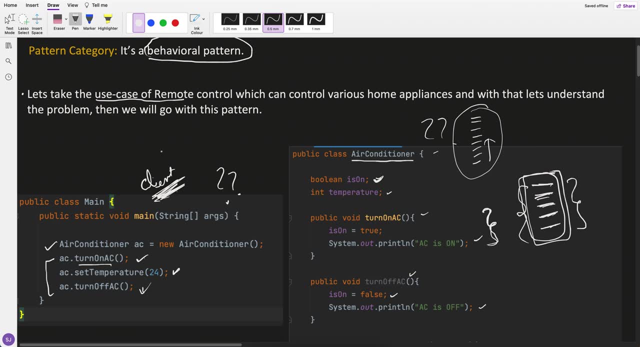 what if I want to implement the undo redo capability, how it will be handled, with client going to handle it? If yes, then that's a very, very bad design If client has to keep the knowledge about what all command it has, what all command and the sequence of commands it has given. 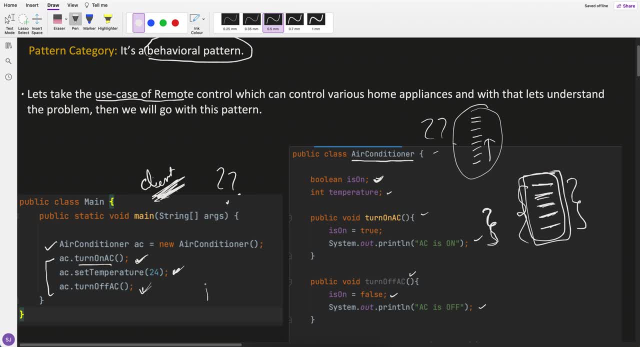 And whenever undo has been done it has to do in the reverse order. So client never should have knowledge about this. it just give like: okay, I need to do undo, then who will do? will air condition will do? no, air condition is a dumb operation. like dumb object. It's like. 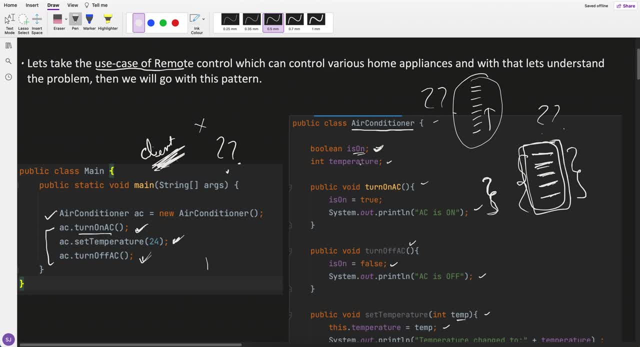 on. if somebody will say, Hey, turn on, it will get turned on in. somebody will set the temperature. it will get temperature. why it will take a responsibility to do the undo operation. So who will do So? in this design I would also see a problem of undo redo functionality. it's very 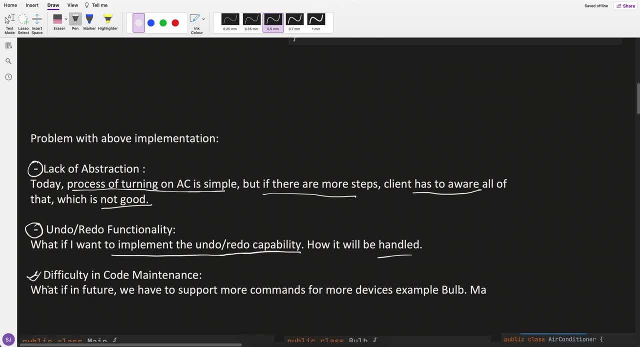 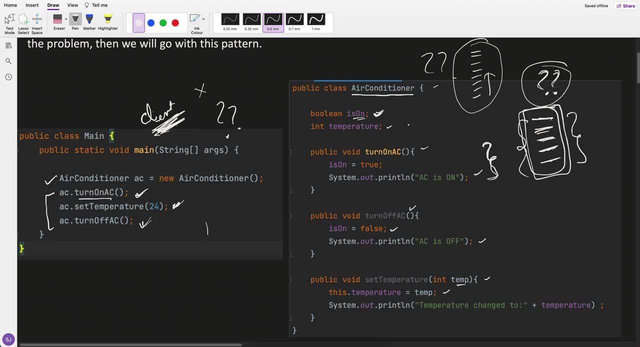 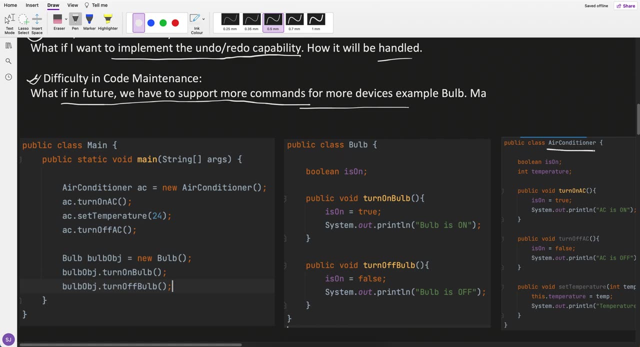 difficult to implement. The third one is difficulty in code maintenance, which I see. So what if in future we have to support more commands for more devices? So let's say today we have air condition. let's say we have another called bulb, So today was only air condition. let's say I have added another. 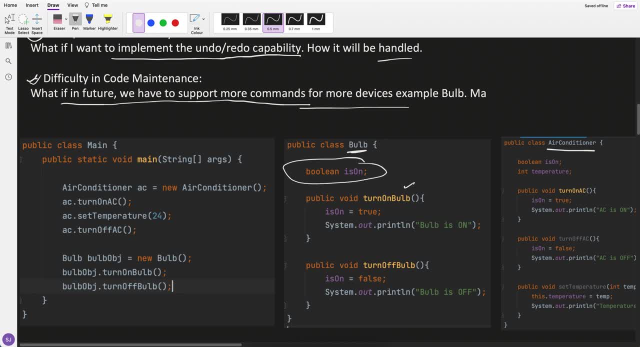 bulb. So bulb also has something. all is on. turn on bulb, turn off bulb- right, So does. client should have no air condition functionality, then it should have a bulb control functionalities. turn on the bulb, turn off the bulb- right, So that become code. 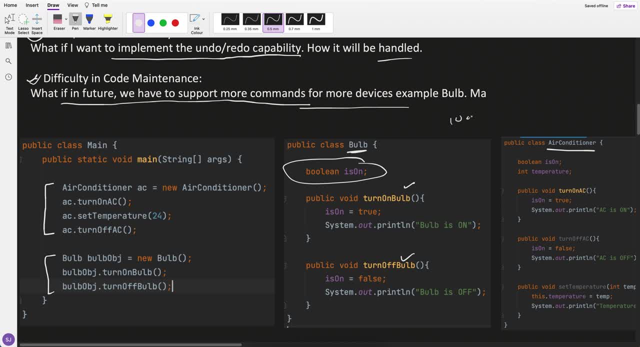 maintenance become very, very difficult. If there are 100 devices will now client will become has to know about all the 100 devices also right, so it becomes become very, very difficult in code maintenance because your client will become very, very bulky and very, very tight coupled. 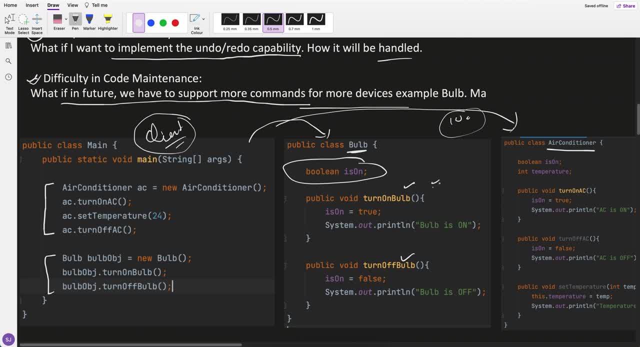 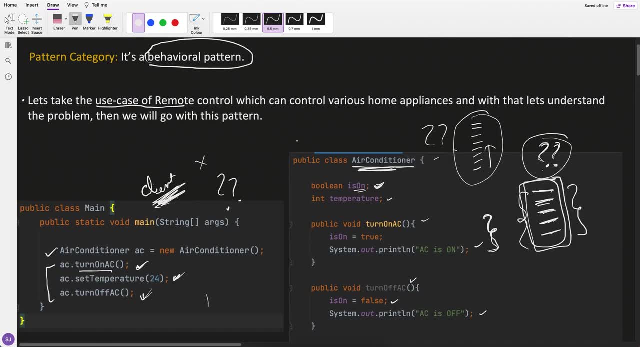 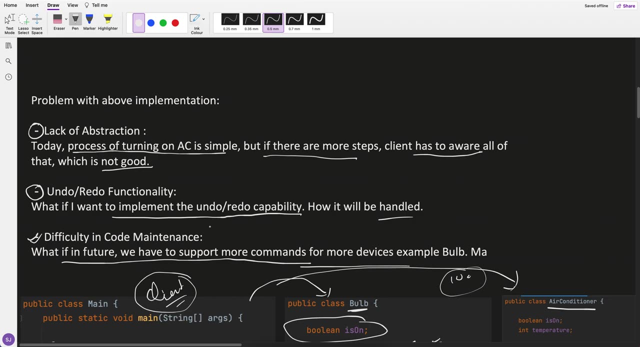 with these objects Right. Anything got changed into this client will get impacted. So these are the three major issues which I see Today. it might not be an issue Very simple, but b 8, 7- these three- in future development it might cause an issue. Okay, so now how to resolve. 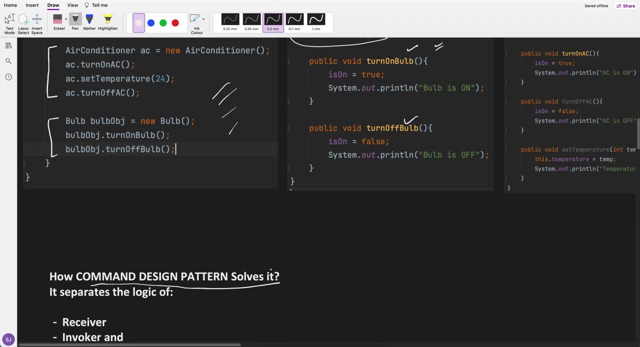 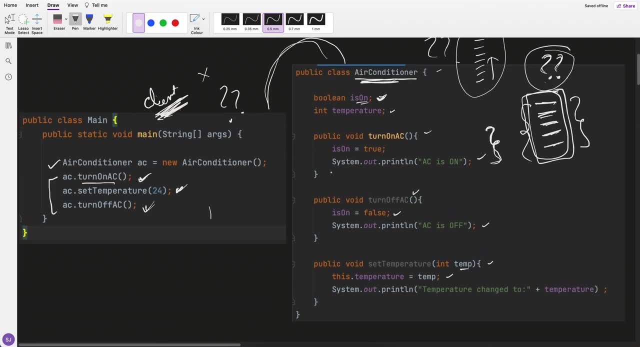 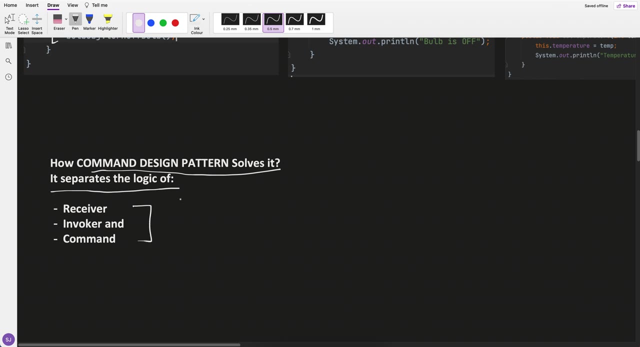 it How command design pattern resolves it. So what command pattern does it? it divide the logic into three parts. So there is simple in this simple layer, condition and client. it divide, it identify the three things: Who is the receiver, Who is receiver? So it put: 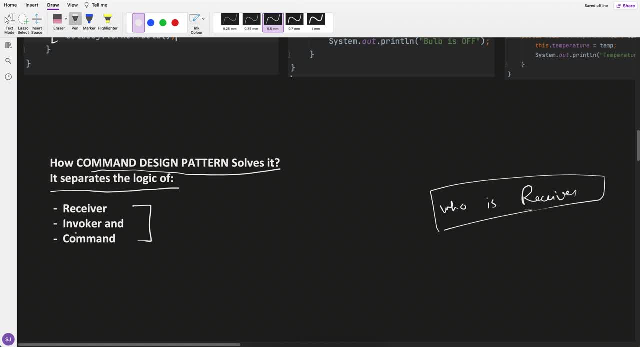 receiver code into the receiver class, Then invoker: who is the invoker? He put the invoker related code here And there is something called command. Okay, so now invoker generates a command and this command is intend for particular receiver. Okay, so now your client use this. 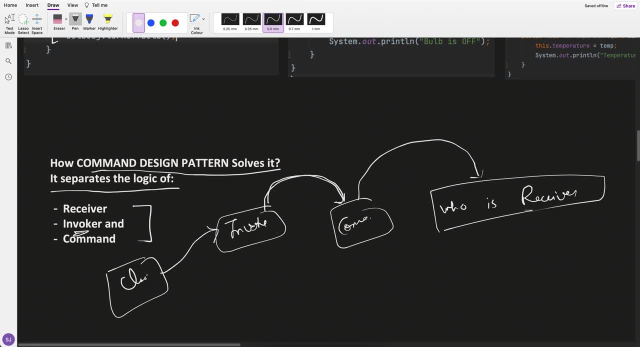 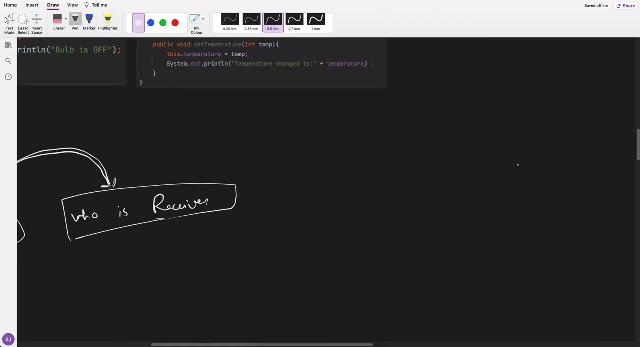 invoker to generate a command which is intend or control a particular receiver. For example, take this your TV. So TV is your receiver, Right, This is your remote control. This is actually your invoker remote. This is TV, which is a receiver. This is a. 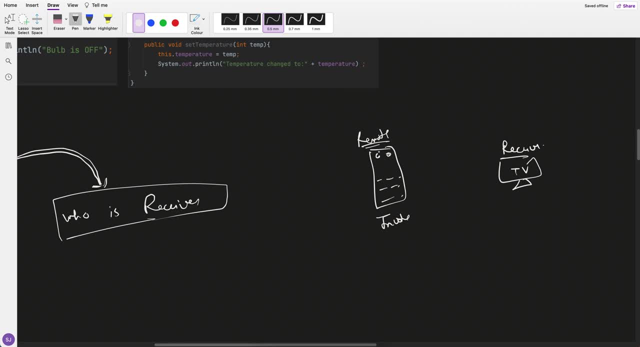 remote, which is actually your invoker Right, And this is, let's say, a remote control, And this is, let's say, a particular client which use this invoker, which use this invoker to generate a command, and how the command will generate whenever it press a particular button. 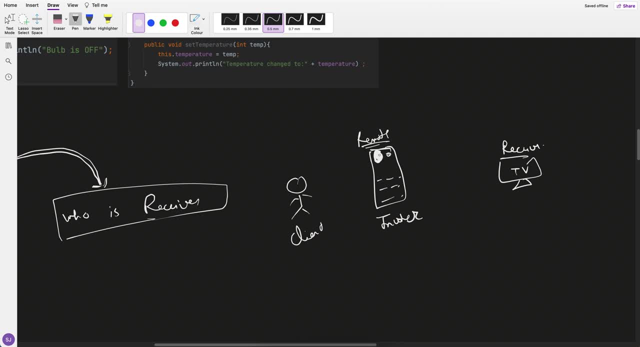 whenever a particular button is pressed. a particular button is, you can say that it will generate a command. it will generate a command to the receiver. Okay, so there are four things: client, invoker command and receiver command- receiver. so in the command design pattern it try to identify this four things. 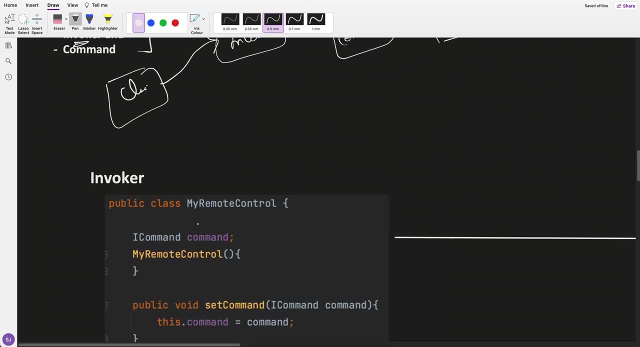 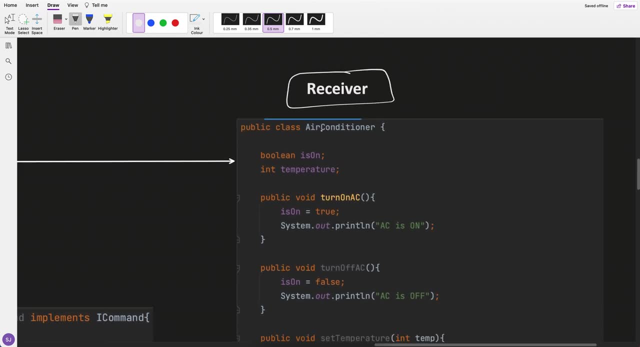 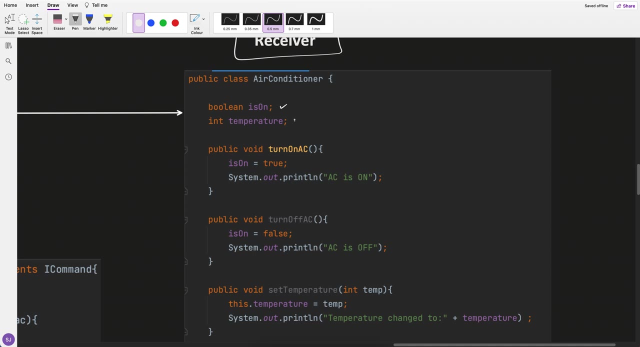 so now let's see this, the same example, air condition, with the command design pattern. so first of all, let's see this: the receiver. so air condition. I told you it's a receiver, so it's the same example I have used as the above. it has two things is on temperature. 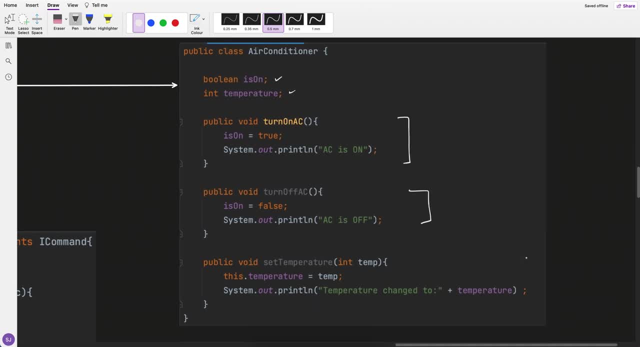 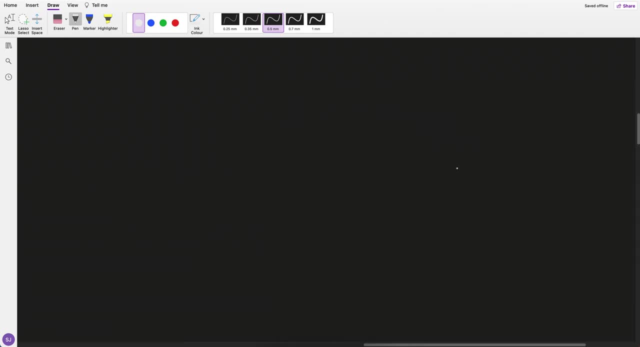 I have a method: turn on AC, turn off AC, set the temperature right. very simple: this is a receiver. okay, then what I need was this: this command. so invoker, use this command to control the receiver. so there is something called now command. this is the second part. 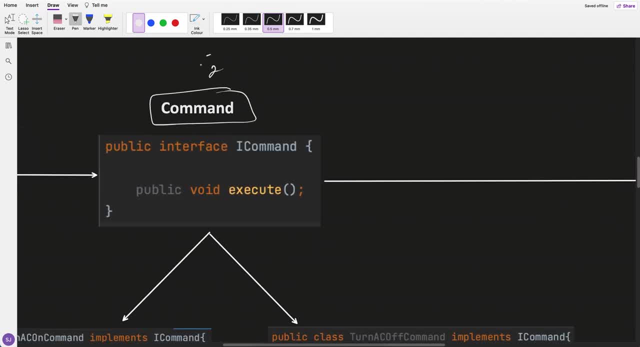 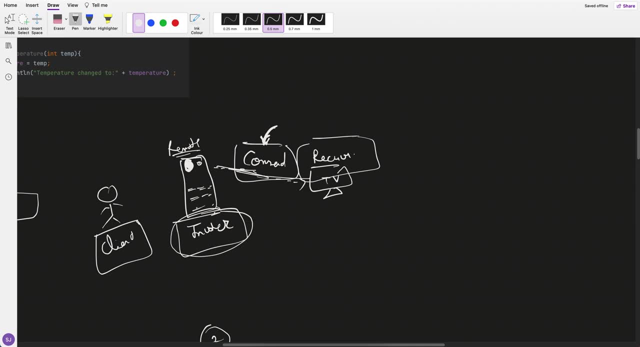 is command. so this is your first part, receiver. second part is your command. so in command there can be multiple commands. it's not like so. remote has, let's say, 20 buttons, so for each button there could be a different, different command. let's say so. I have created an interface. 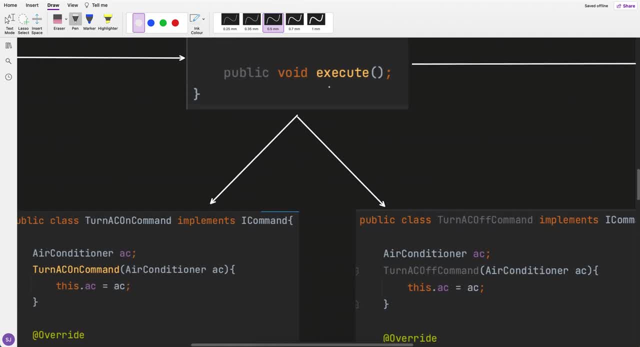 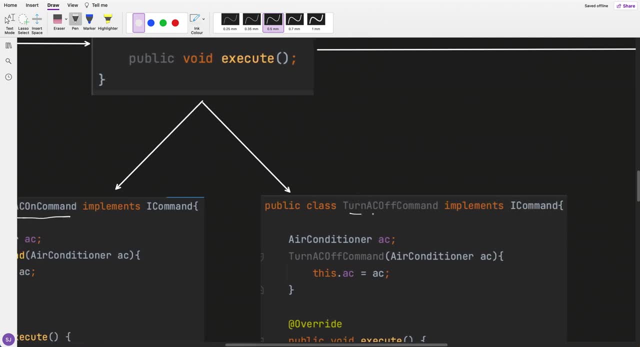 interface command. I command right and I have put one method execute. so I have created different, different command: turn AC on command, turn AC off command. similarly, you can put another, let's say set temperature command, right, Okay, Just I'm saying what all different, different things can come. you can put other, different. 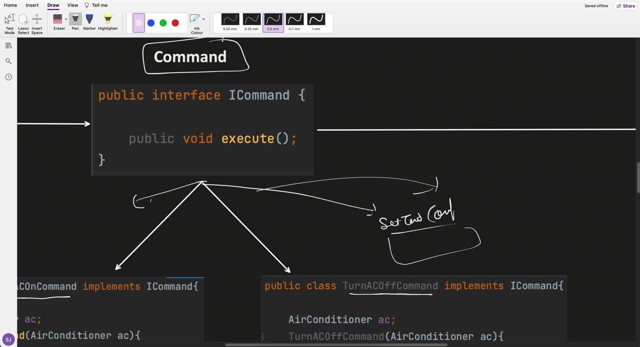 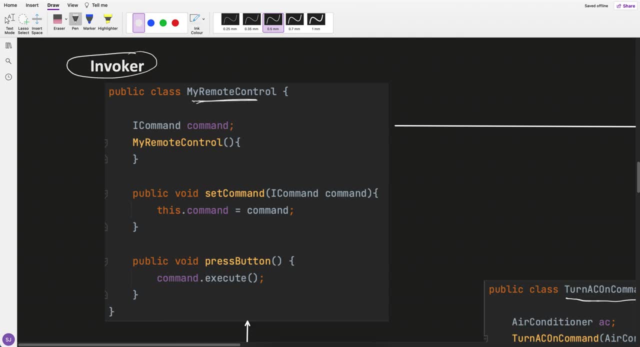 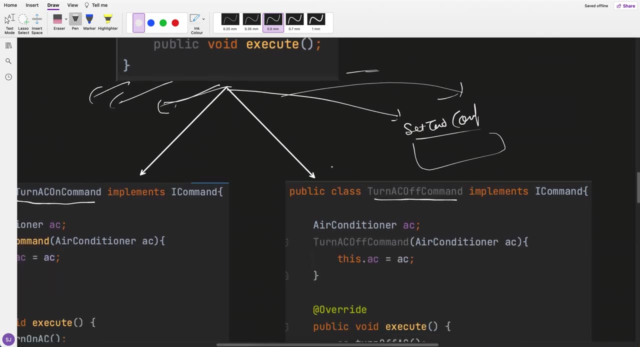 command with one remote control, with one like what. all commands are possible through one invoker. so this is your invoker like a remote. so one particular invoker can generate what all commands. you can put it here. expand it: there could be 20 command, 30 command, 40 command. 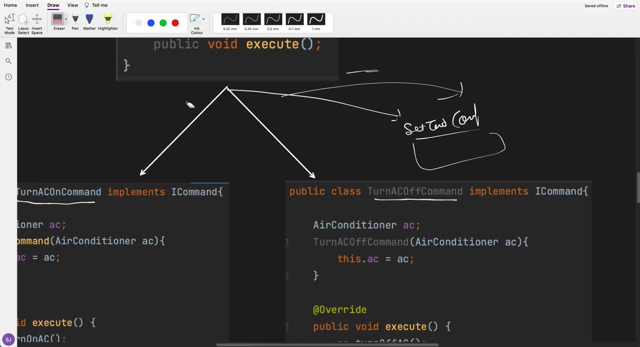 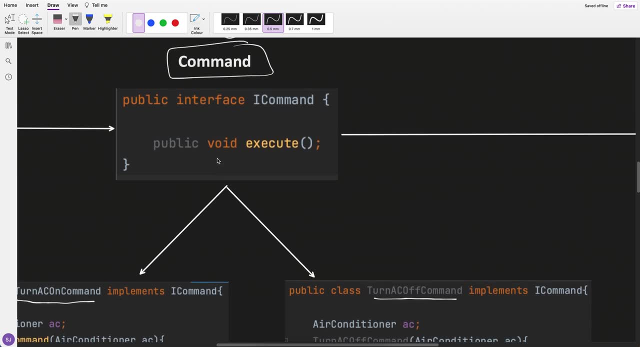 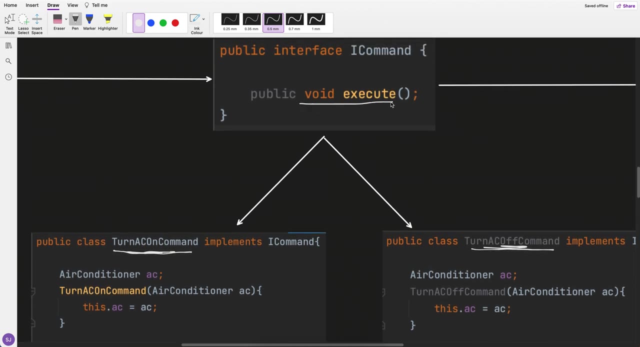 no matter what, whatever the invoker can generate a command, you can put it here, Okay. But let's say, for this example I have taken, that only two commands are possible: turn AC on command. turn AC off command- okay. so this is an abstract method. so both the classes. 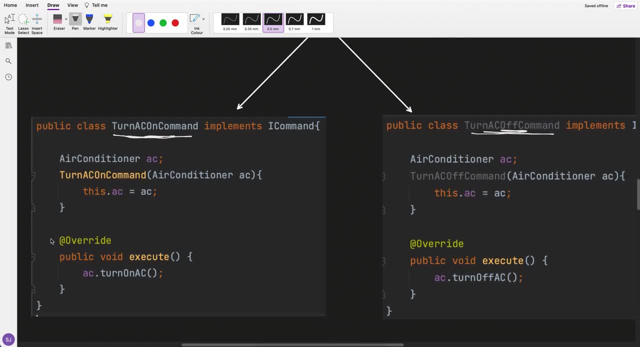 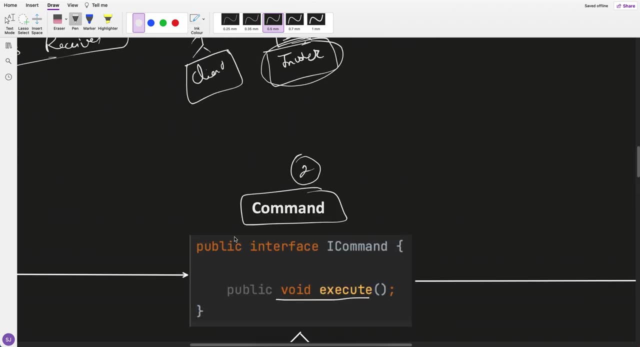 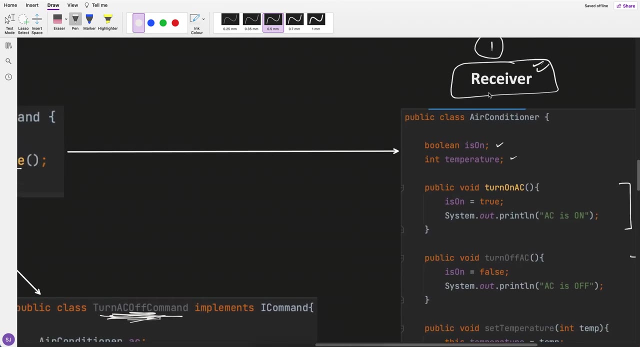 concrete command class has to implement the this right. so here, if you see that they have an object of what receiver- so that's why I put that- the concrete command class has to has receiver right. so here we have an AC objects or this you, I am using the constructor to 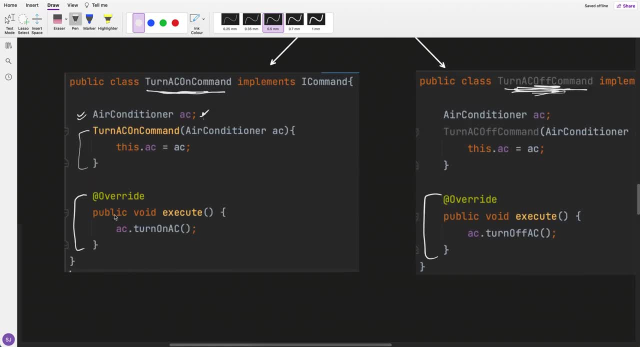 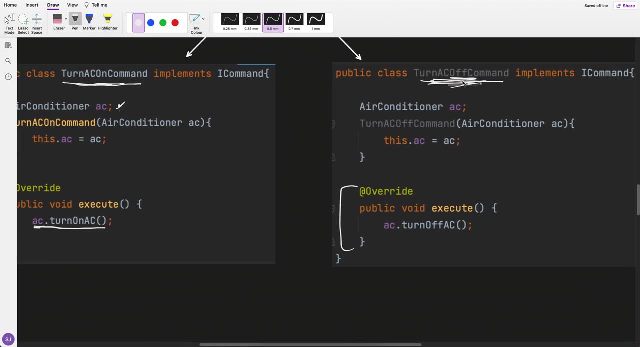 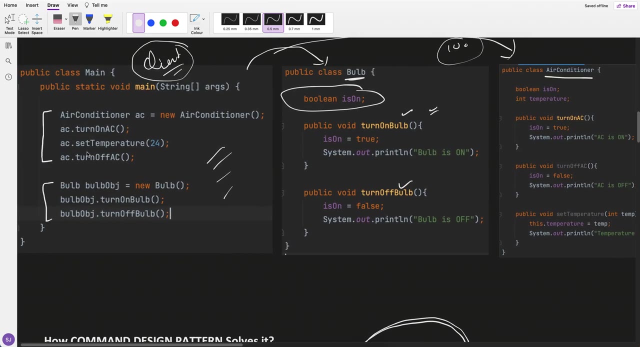 initialize this object right. so now, but this is the main part. so here I am using this AC dot turn on and in the turn off command what it is doing, calling the method turn off. so one thing: you might have noticed that what we have done is so this turning on, logic turning. 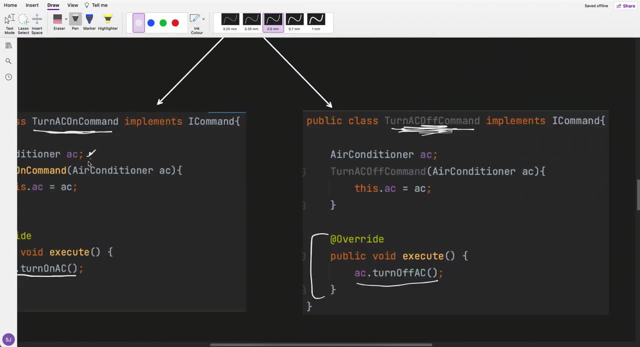 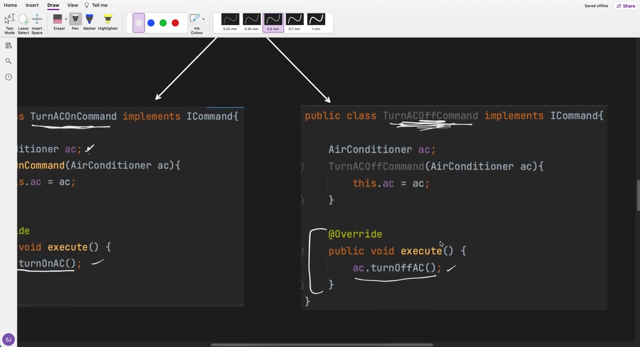 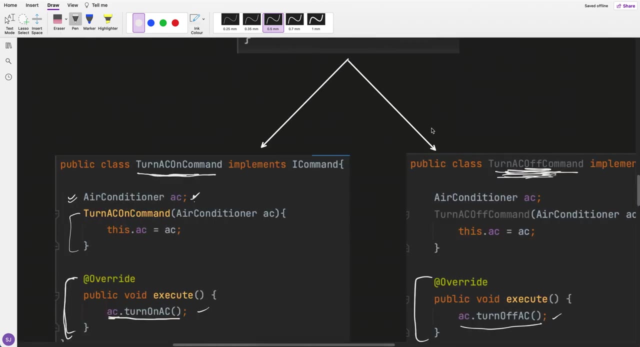 off logic. I have put up in an appropriate command class right today. it is very simple, but maybe in future, if this get change, only this particular command class will get change. if there is a change in the receiver to do a particular command, only particular command class get. 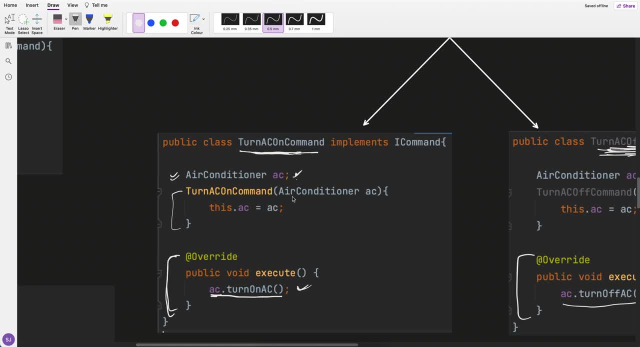 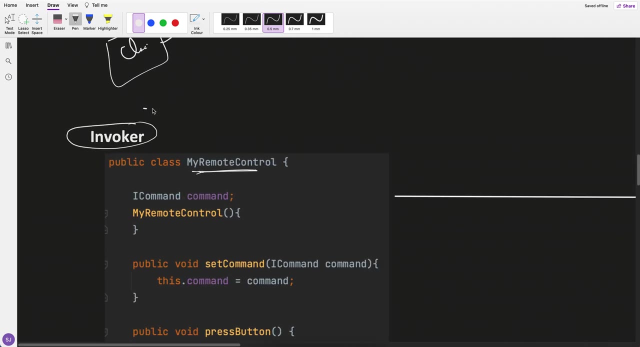 change. if the process of turning on the AC get change, only this particular class, turn AC on command- will get change right. So they have the receiver object And through this they are performing their command. OK, Now this is the third, which is invoker. so here I have my remote control. so I told you. 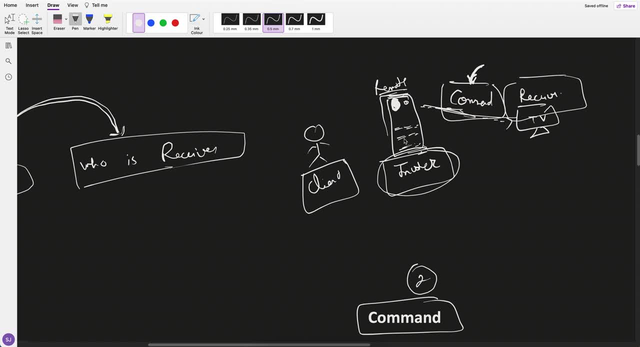 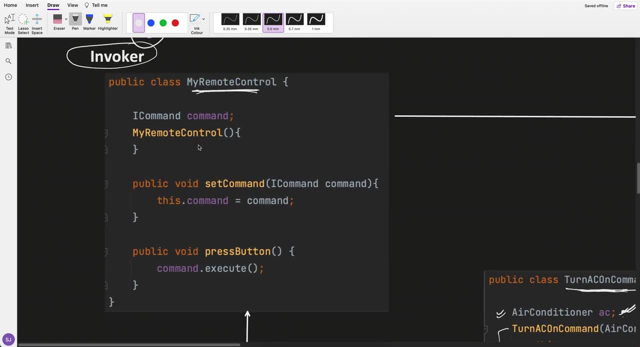 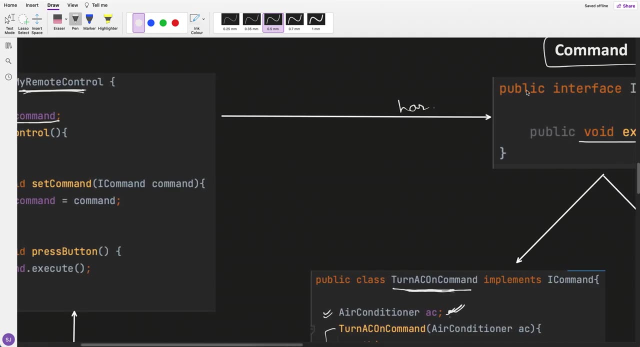 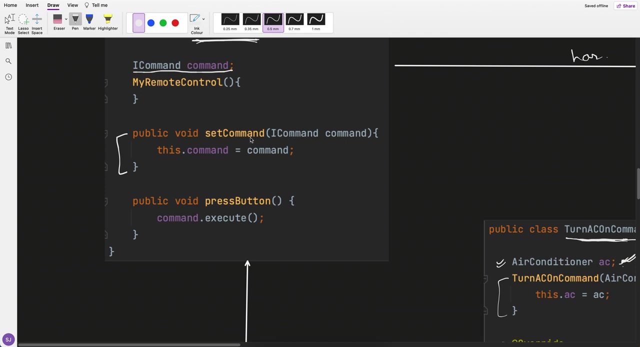 that this remote is your invoker, so this remote has, you can say, that button which generates a command. so they have access to command. so here Remote control has command object. it has, Remote control has command object right. so now I am setting the command. whatever the command, whichever the button client will press. 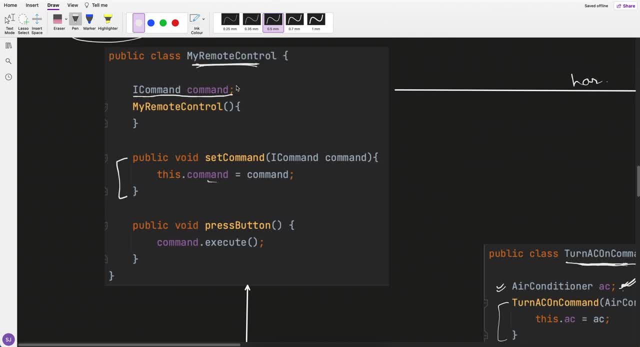 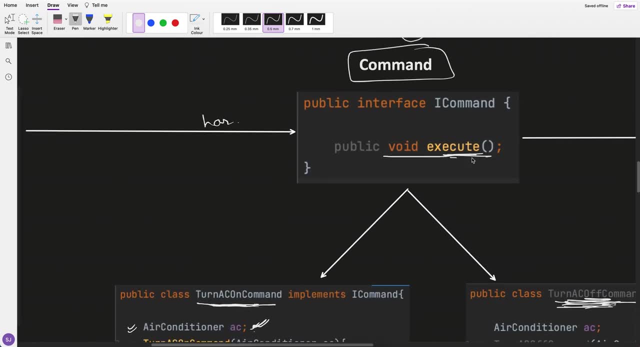 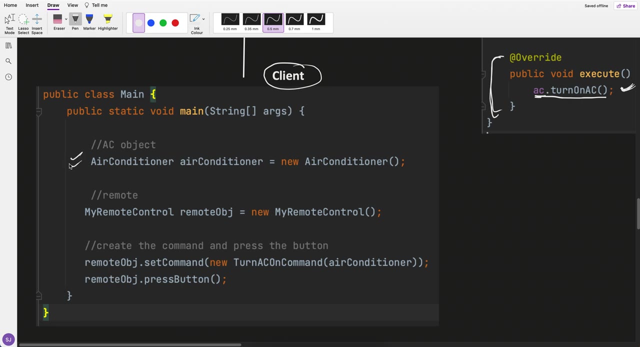 that command will get set into this and whenever the button is pressed, what it will do is command, dot execute, command, dot execute. okay, so it will make sense with this now. now let's say: this is the client. so first I am creating an object- ac object. so let's say ac got exist, then I am creating 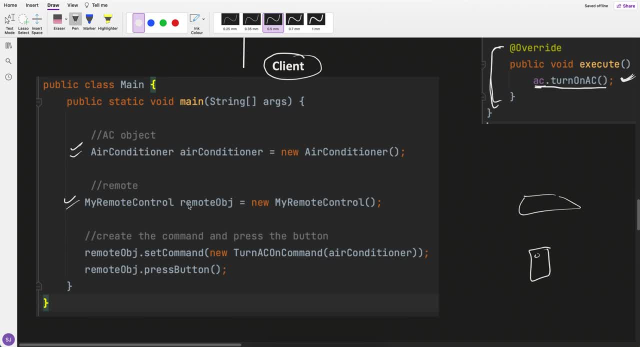 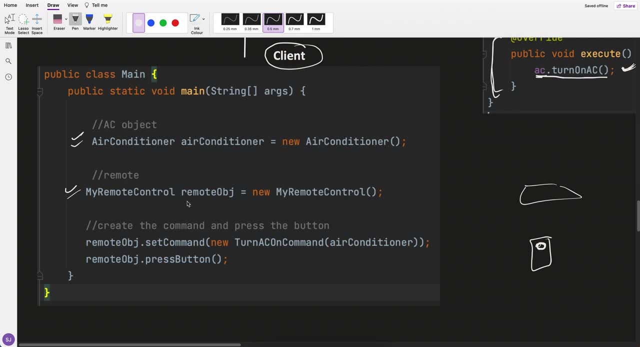 a remote. let's say remote now, remote exists. now what I am setting is: so let's say there is one button, understand that remote has only one button, right? so I am the remote object. I am setting a command. what is the command I am setting? turn ac on command. okay, so in the remote control I am: 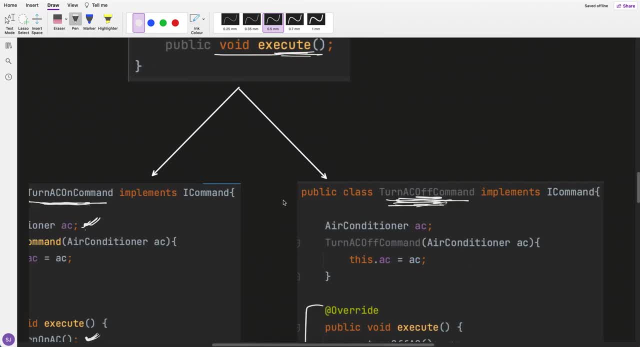 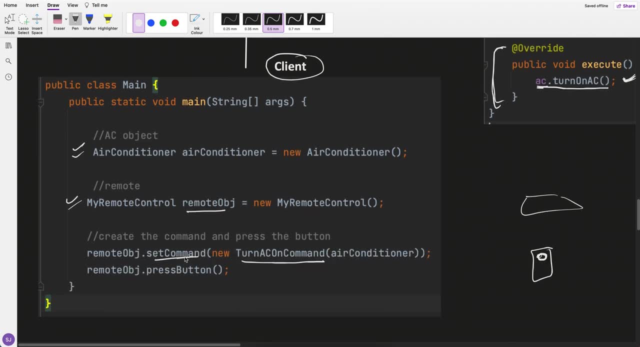 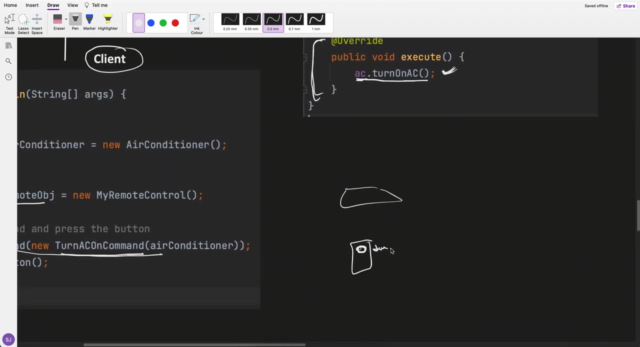 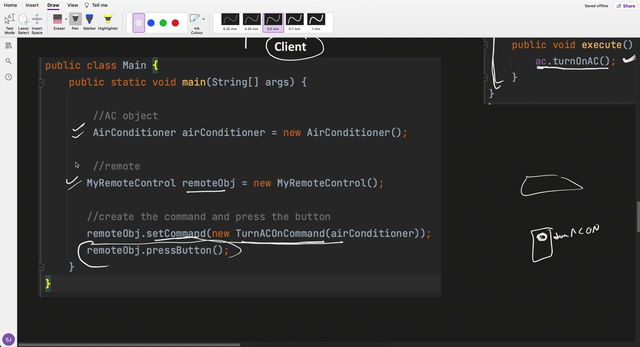 setting the command. what command? I am setting one particular command, right, let's say, I put turn ac on command here, so this command has turn ac on command. AC on command. so I have set the command here turn AC on command. okay, so this is: has the turn AC on button now. so this is the real code of the object. so till now what I have. 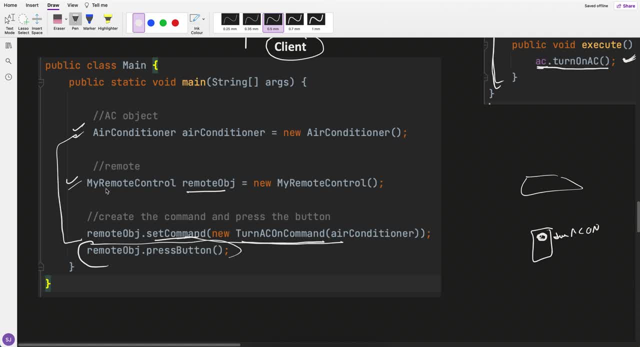 done is: I have done a setup. I have a setup for the AC. I have created the remote. I have done the remote has a button which internally might be. I have set up the turn on AC command. okay, so now this is actually what clients are interested in. client will just simply. 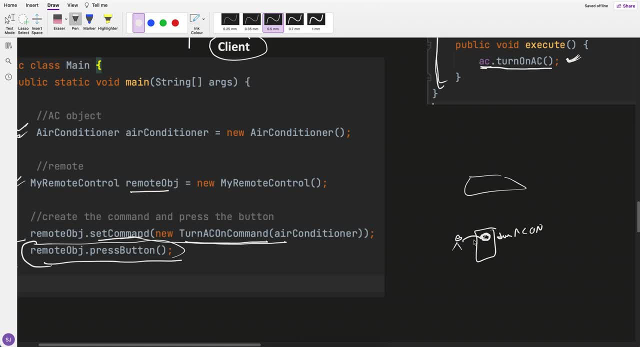 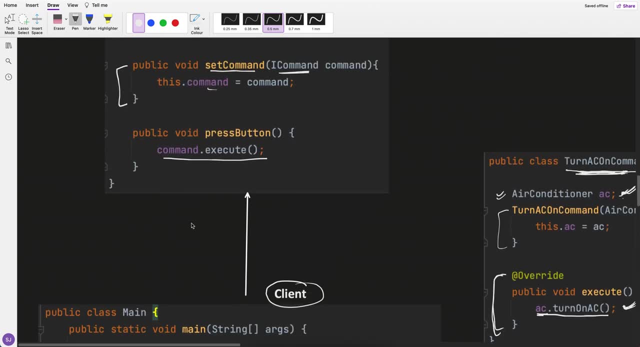 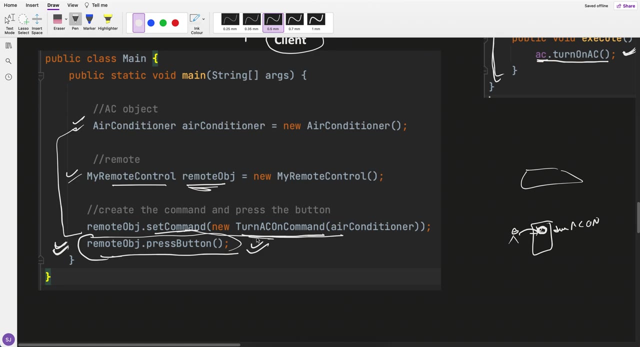 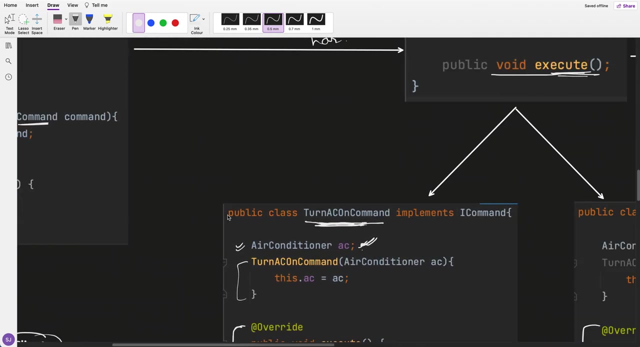 press the button. so now client will simply press the button. press button. now what will happen is remote object: my control. press button so this method get invoked. what it will do? command: dot execute. what command it has its this button already has turn on AC command set right. so turn on AC command and so it will call: dot execute. turn on AC command and. 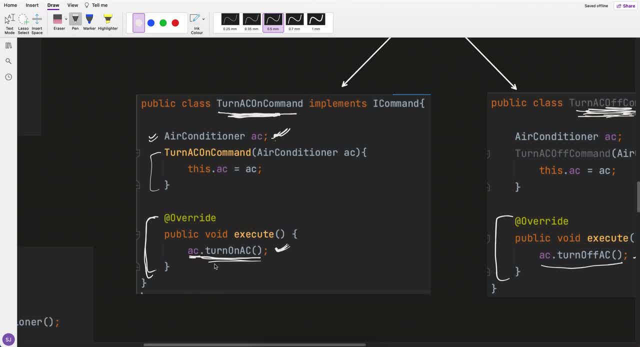 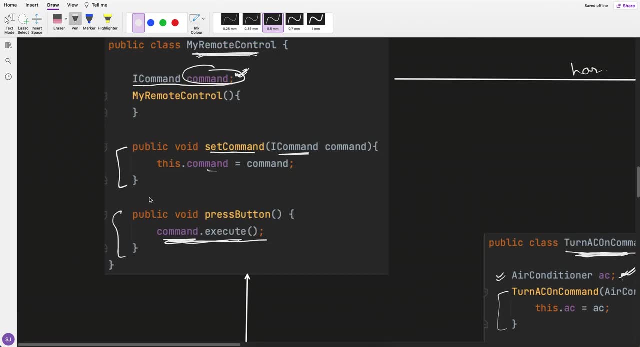 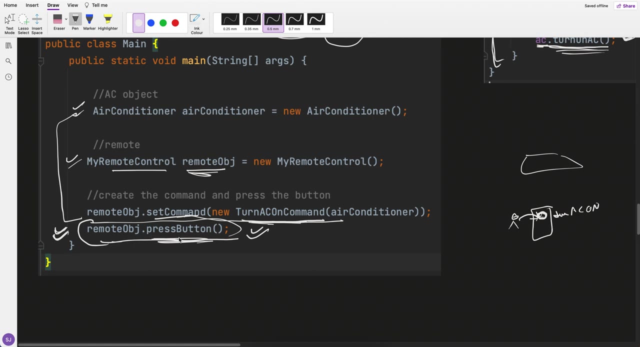 command execute. it will turn on the AC. it will change its status. okay, so now here, if you see that the client here, the client doesn't have to worry about it, all have to worry about press button, that's all. it doesn't have to worry about anything. this three line of code set up AC. object: remote: this is you can. 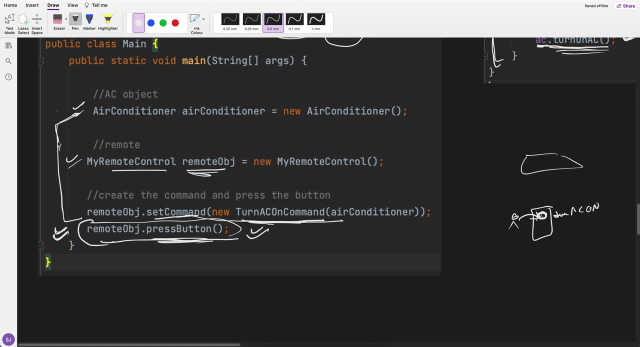 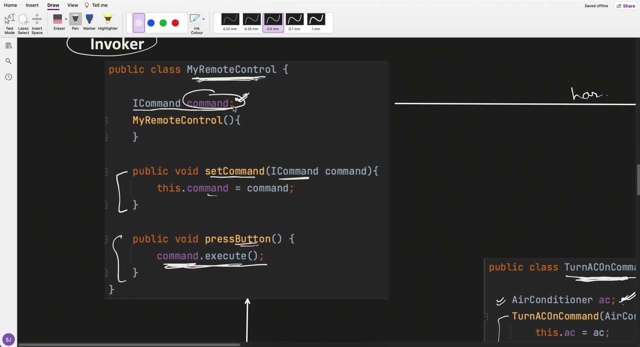 say that for testing purpose, we have to create, we have to create an AC, we have to create a remote, we have to create a button for that one right, but all client has to do is press the button. once it press the button, the in the remote control, when it press the button, a particular command will be used to invoke. 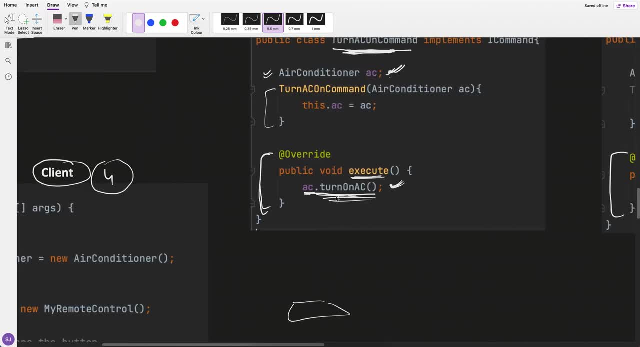 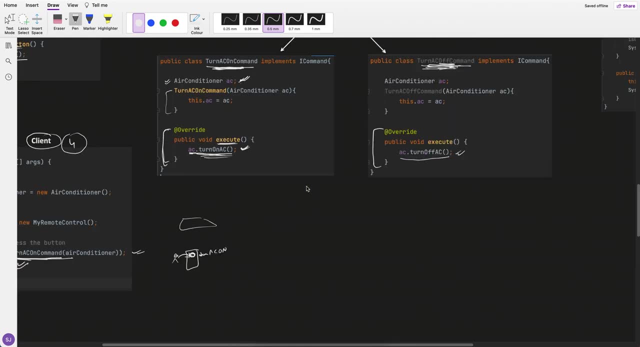 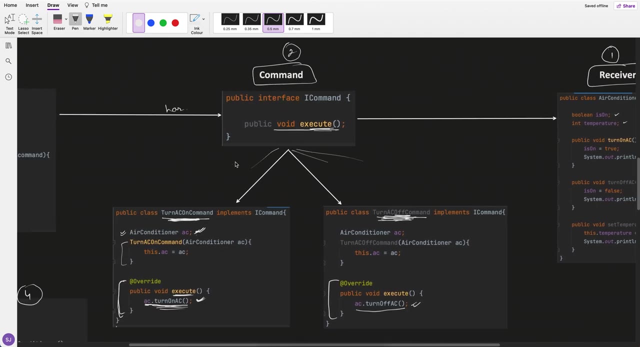 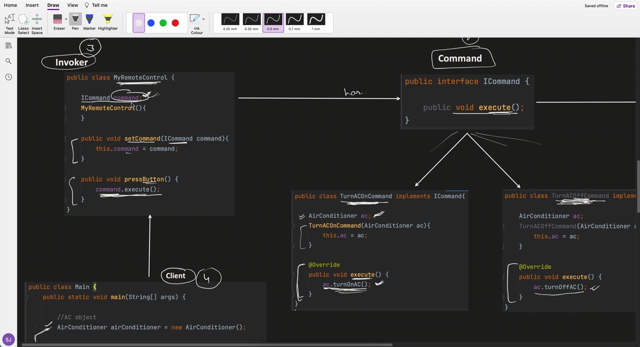 the receiver particular method. okay, got it. so this is here. if you see that first is receiver, then second part is your command. you can have any number of commands which is supported by a particular invoker, then invoker have command. let's say press button option which invoker? 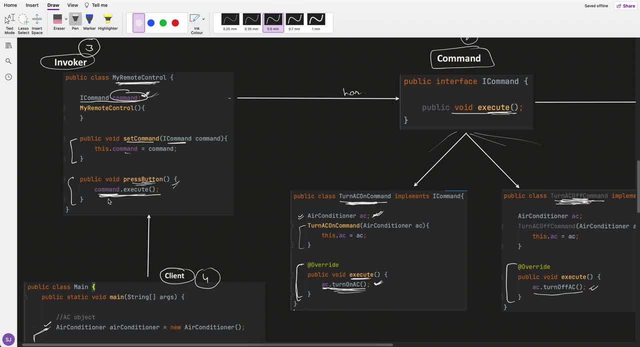 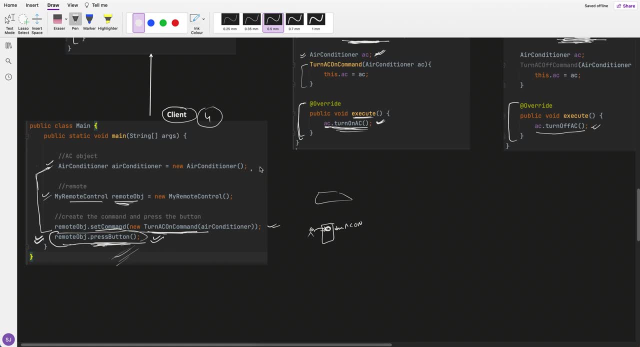 has the command right. so whenever a button is pressed, a particular command will get executed. client has all has to do is press the button, and this is just a setup which we are doing it so whenever a button is press up. so in this button or in this command, whatever the 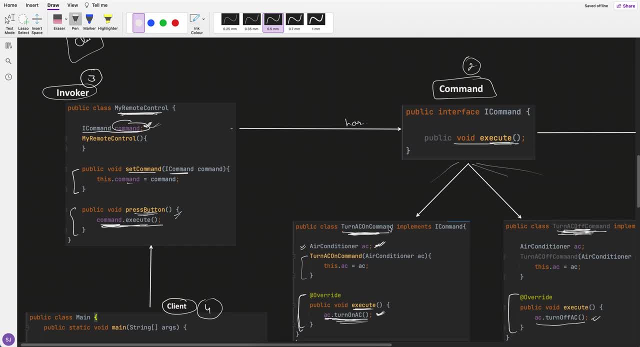 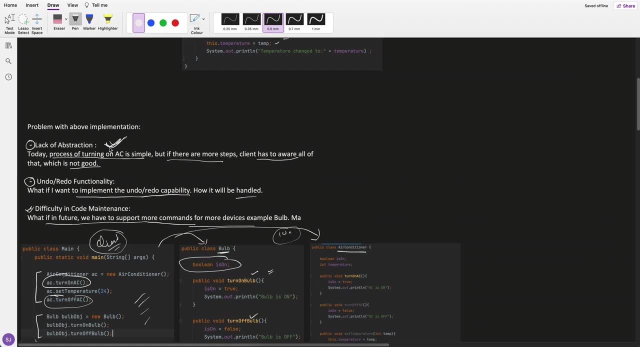 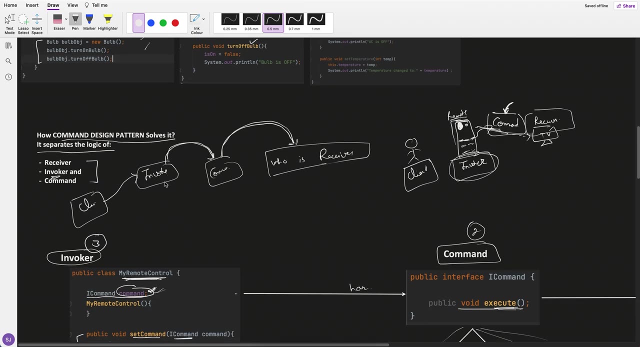 command we have set, it would be used to invoke a particular command. ok, so now till now, we have resolved the lack of abstraction part right, and also the difficulty in code maintenance is also resolved right, because let's say in future a bulb as the same remote is used to. 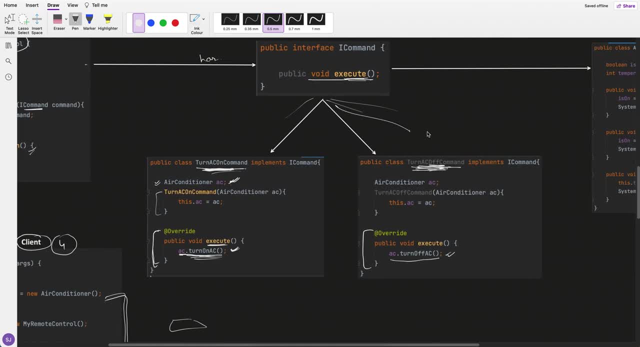 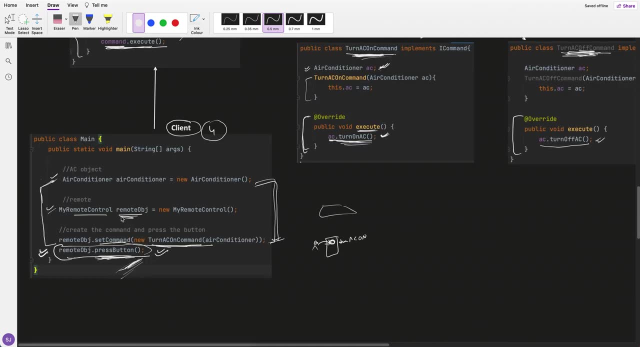 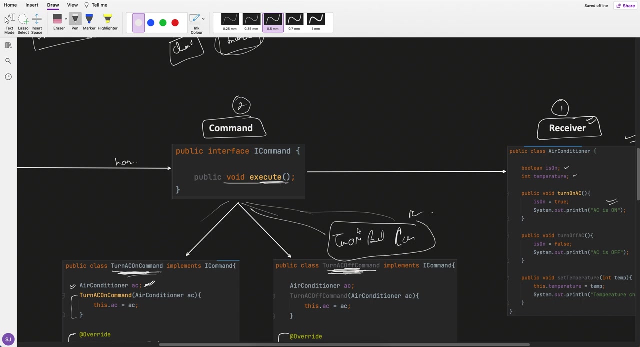 control the bulb also Right. I can have one method like turn on bulb command. turn off bulb command right. so on a particular press button right, what command I will pass? turn bulb on command right. first I will set the command and then I will press the button so that particular command will. 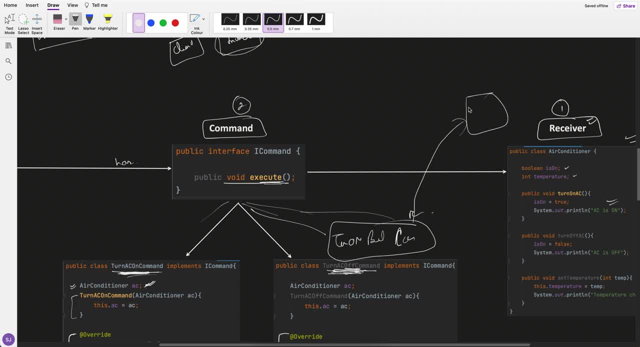 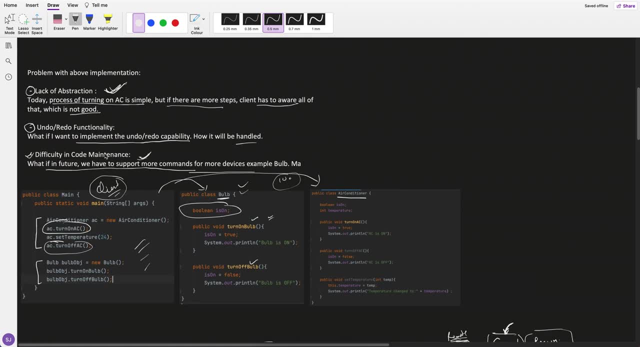 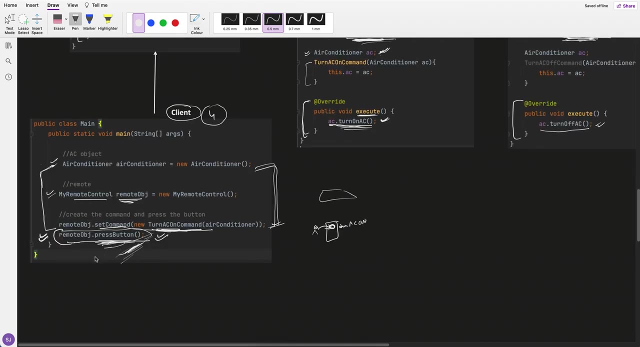 get initiated and that will work on a particular receiver. may be bulb receiver. Okay, so code maintenance is simple. lack of abstraction. we have resolved it with this one, because now client only has to worry about press button. currently, in this example we have only used like. like there is only one button, but we can have multiple buttons for 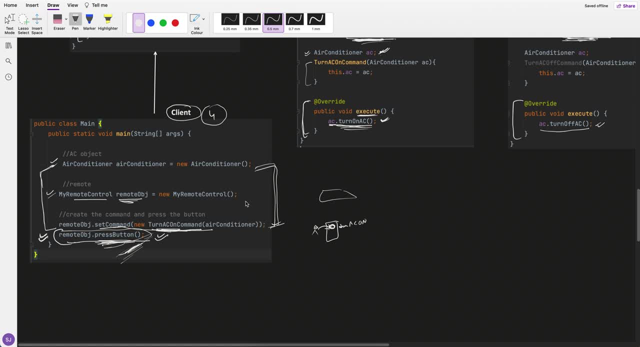 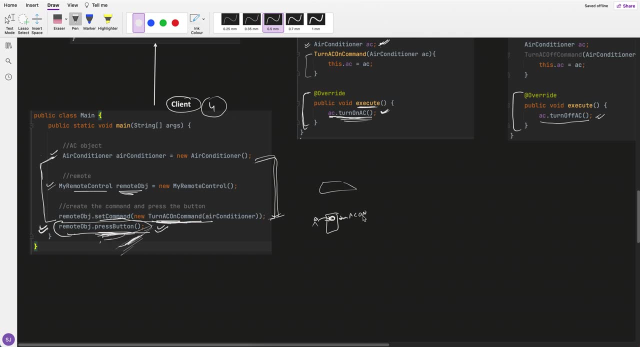 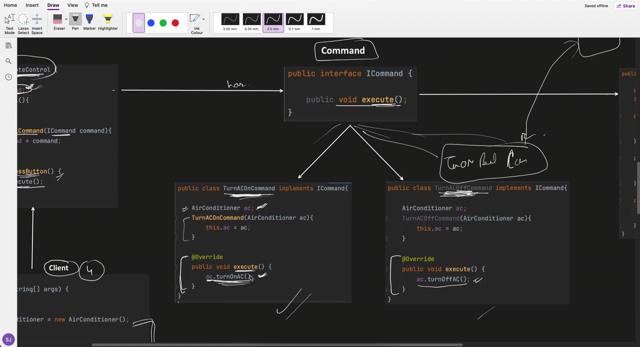 each button we can set a different command and it can be used to perform operation, multiple operations, right. so that is now easy, that any change in a particular behavior of a receiver, Only that command will get changed right, or that class will only get unpacked. now the 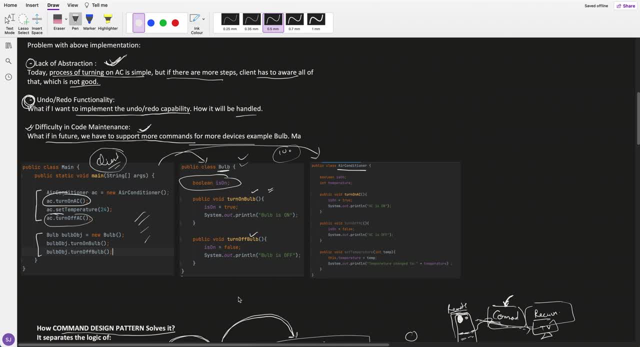 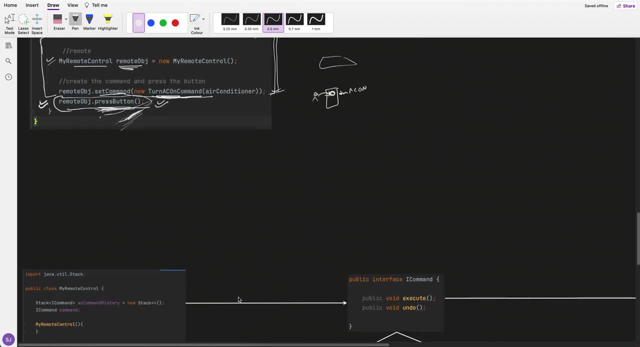 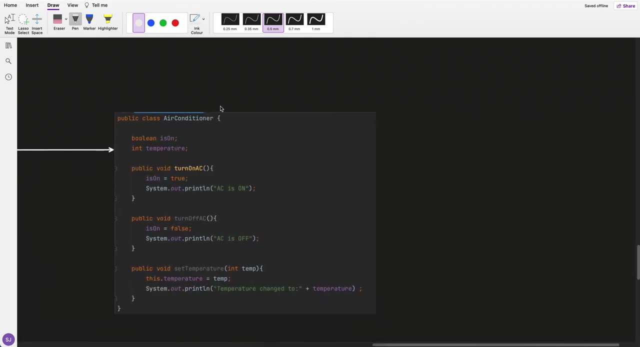 question comes is: hey, how you will perform the undo redo functionality. let's say, interviewer has asked me design the copy paste undo redo functionality of a text editor, how you will do it. so I have solved this simple with. this is like the same thing: first receiver is there. 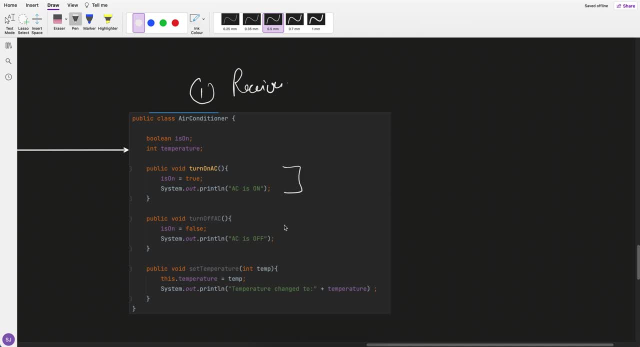 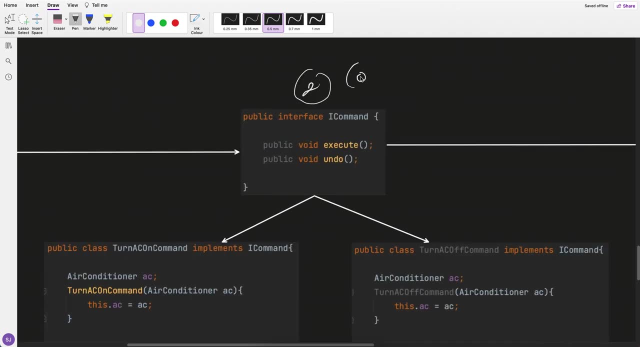 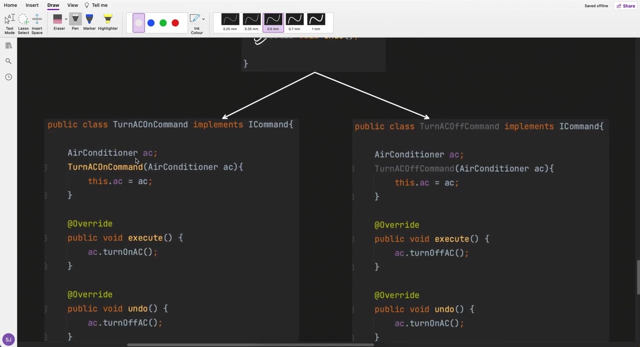 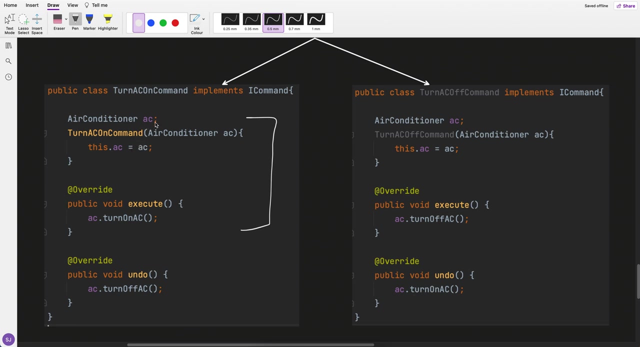 does receiver change? no, it is exactly a same Turn on AC, Turn off AC set temperature. so there is no change in the receiver. second, this is your command. so here I have added one method undo. so for each command, whatever it's, this is exactly same as the previous one I am setting using the constructor to assign the air condition. 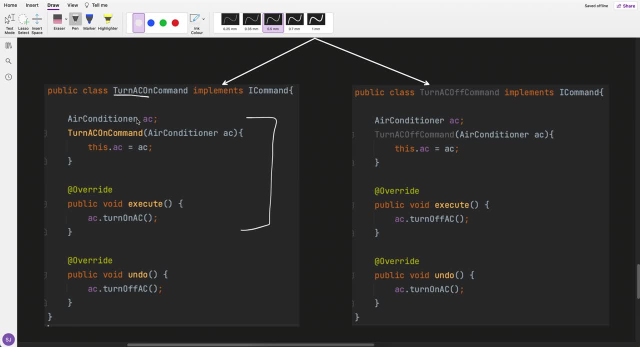 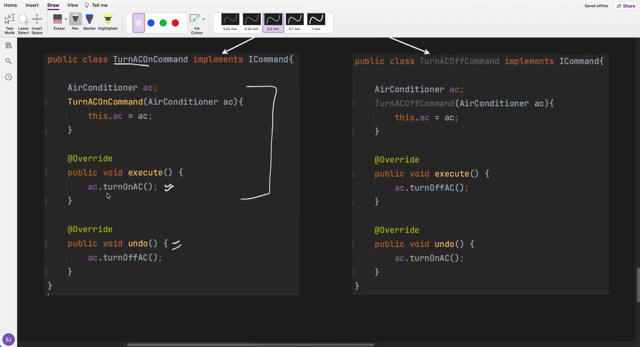 object and in the execute what this command is turn on. so in execute it will turn on the AC. then I have one more method, undo. so what it will do is undo What it has to do. it has to do: turn on the AC. undo in this it will do: turn off the AC. 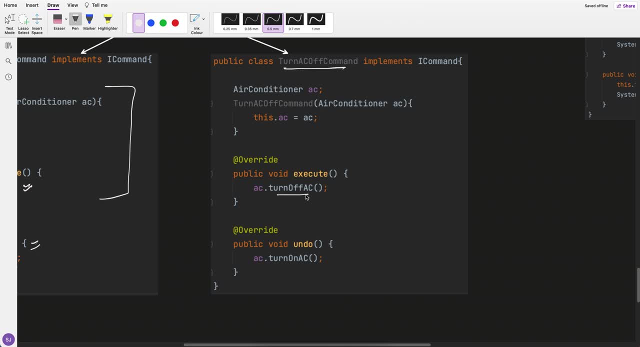 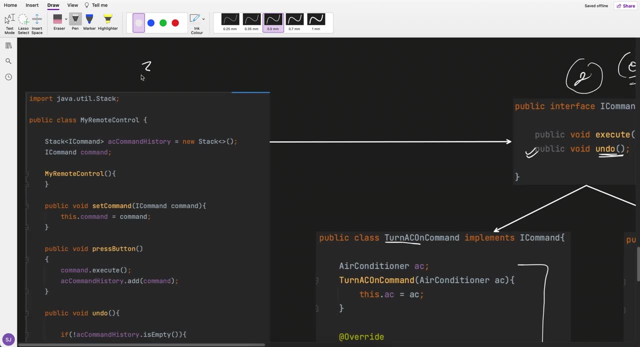 similarly turn off command. what execute it has to do is turn off. in undo it's turn on opposite right. so I have added one undo method here. third is your invoker. so this is your remote control. so here what I have done is because from the remote control, from this: 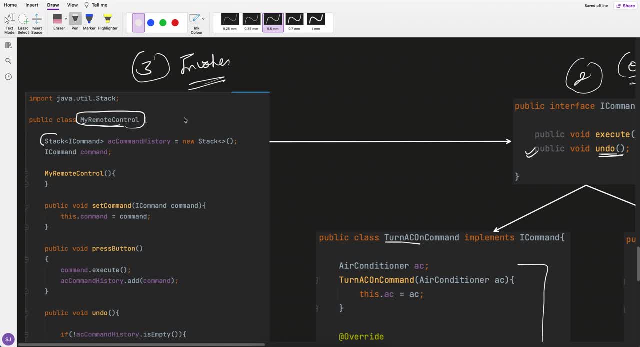 invoker, I will generate the command. So here what I have done is because from the remote control, from this invoker, I will generate the command. So when I press the button I am generating one command right. so here I have used an stack command history right. so now what I am doing is this is exactly same: I will set the command. 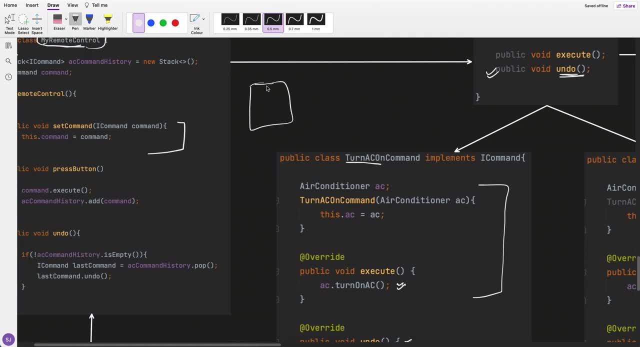 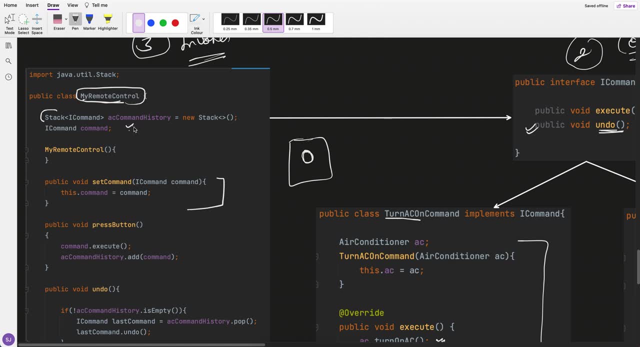 which command I want to invoke. assuming the same thing, a remote control has, let's say, only one button, and whenever you press a particular button, one of the command will get generated, which I will set into here. so I will set the command first and whenever a particular button. 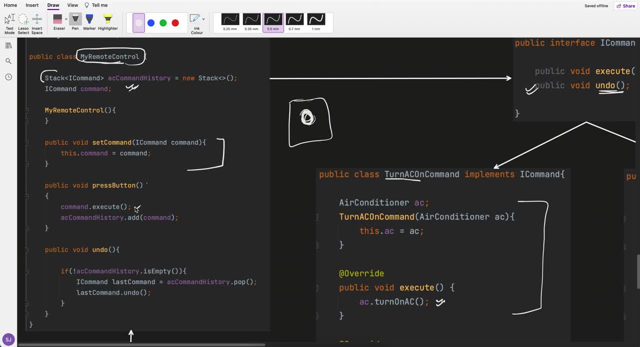 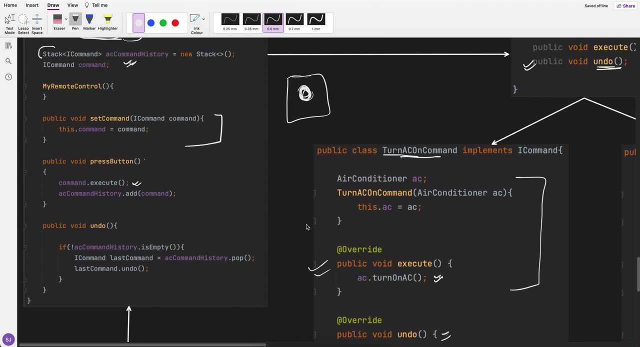 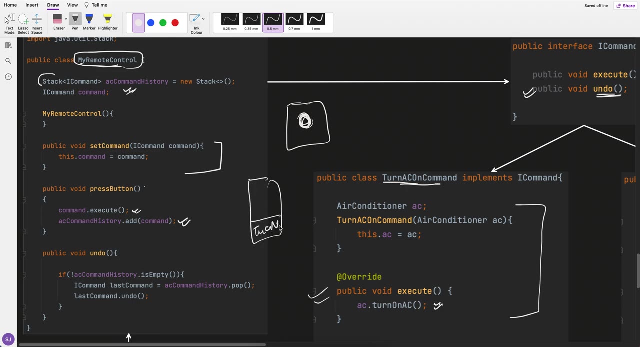 get clicked. Now click press button, it will execute that command. so let's say I have turn AC on command, so it will call its execute option. but I am also adding into an stack a stack of command. so let's say, turn on AC command. second time button press, it will again add into stack. 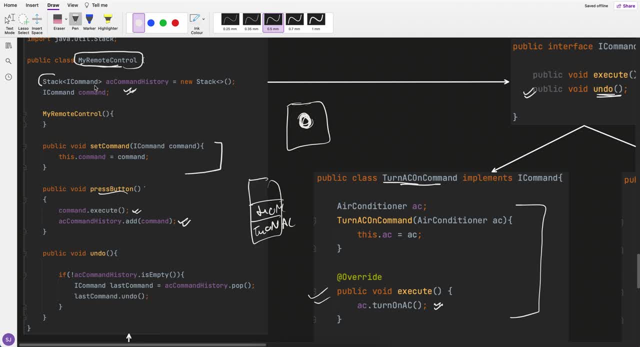 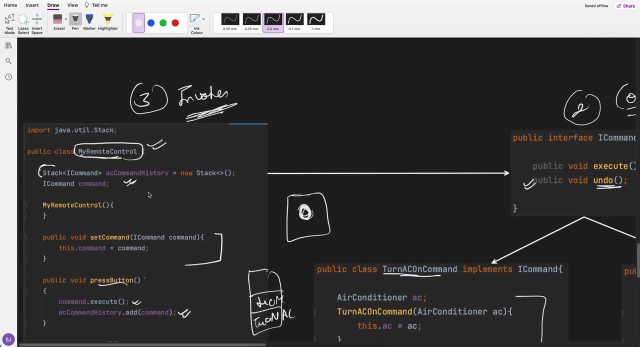 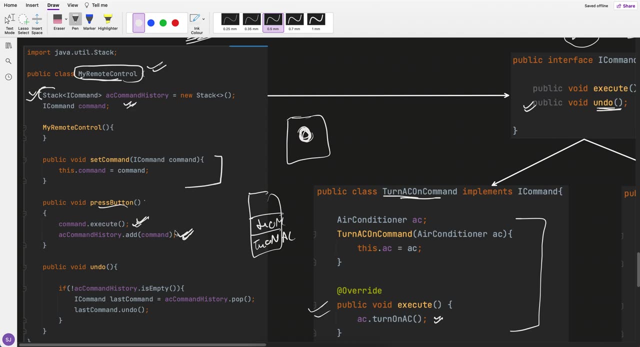 turn on AC, something right. so what I am trying to say is that in the remote control, which is an invoker, Which is the place from where the command get generated, you can put a stack and whenever the command is generated, you can put that command into an stack here. right, and what? 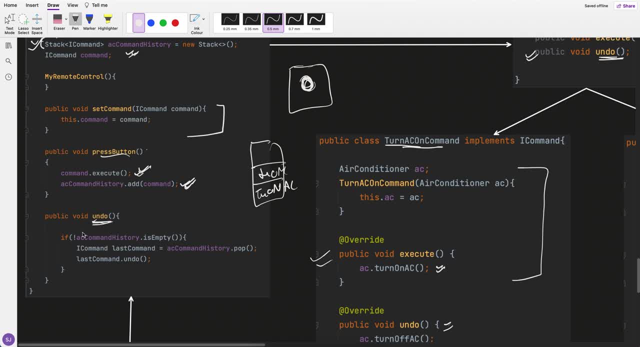 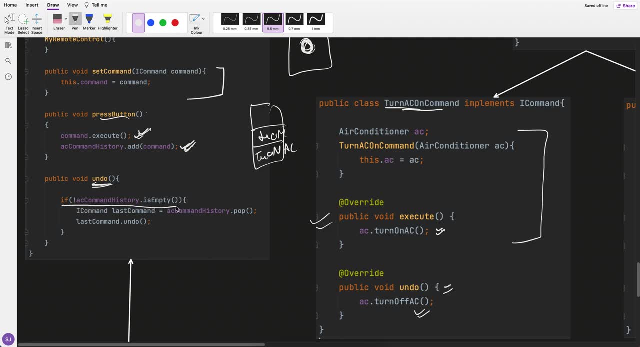 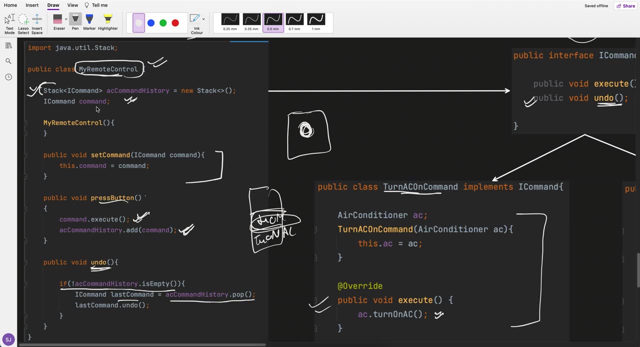 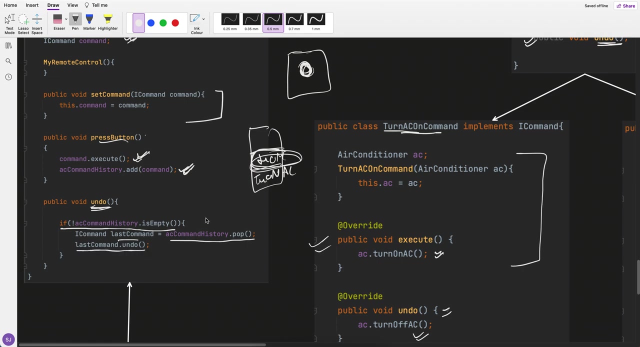 will happen. is it can, we can expose one undo method here in the invoker itself. what it will do is it will check the stack and pop up the last element. so last element would be one command only, right, what? because we are doing different command. So it take out one command and know what it will do. is it will do, call the undo operation. 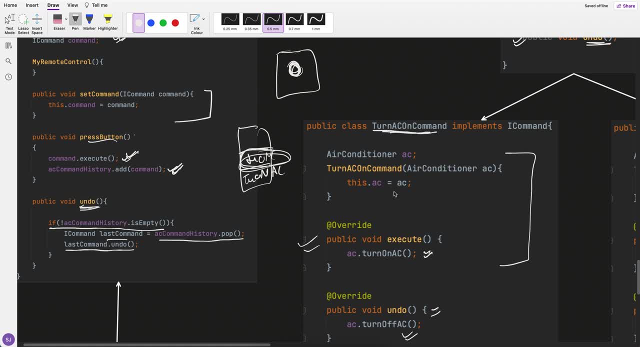 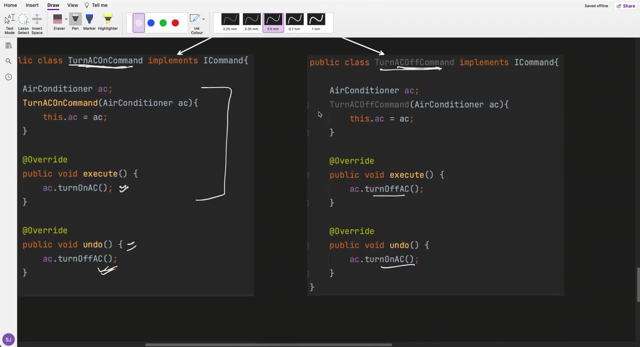 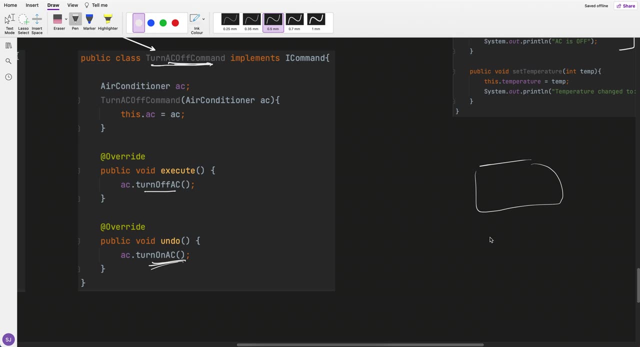 so if command pop out or turn AC on, it will call its undo operation. it will turn off the AC. If the top command was turn off the AC, so it will take out its undo. it will do turn on the AC, right, similarly in the television. you know that right. let's say earlier you. 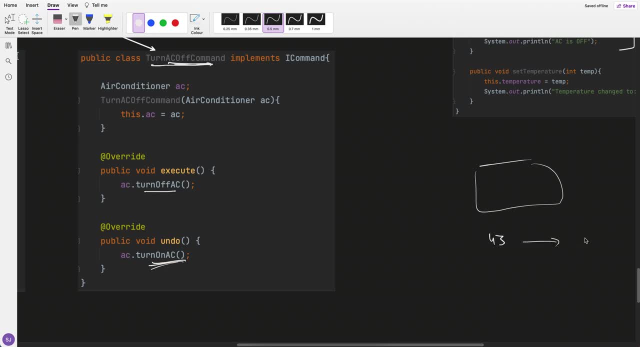 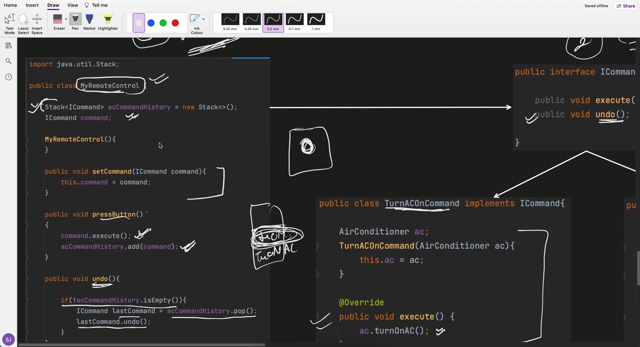 are on channel number 43. You will change it to 54. You can do back. when you click on back, you again go back to 43. what is then? it is like an undoing right so we can easily, easily add the undo or redo functionality also here. right, how? invoker. 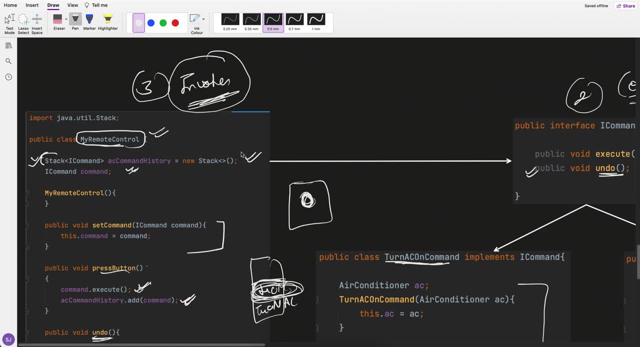 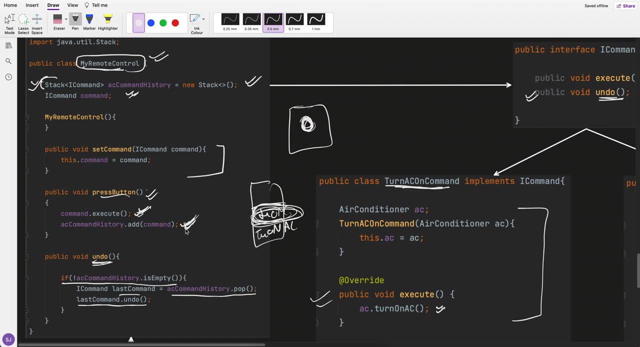 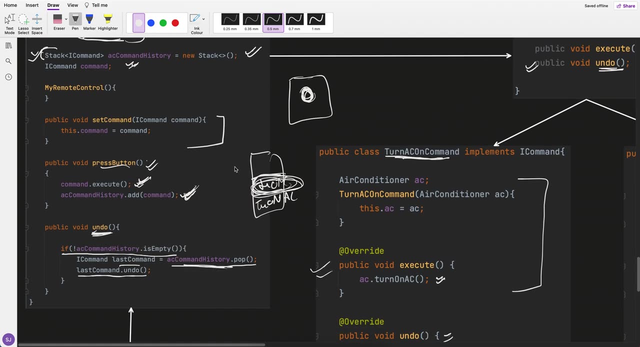 can generate a command. so here we have a stack of commands, and whenever a command is generated during the press button, we can add it into a stack. right, we can expose one method, undo what will take it. it will take the last item from the stack, so you will get a particular. 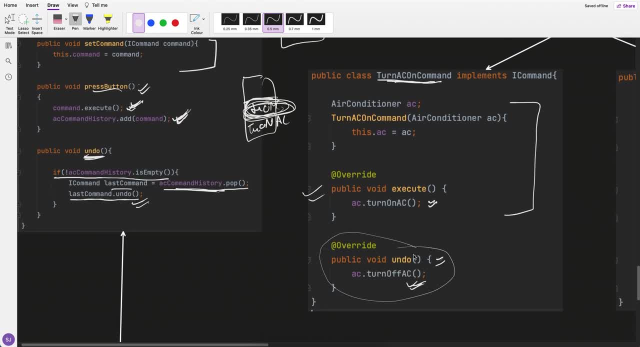 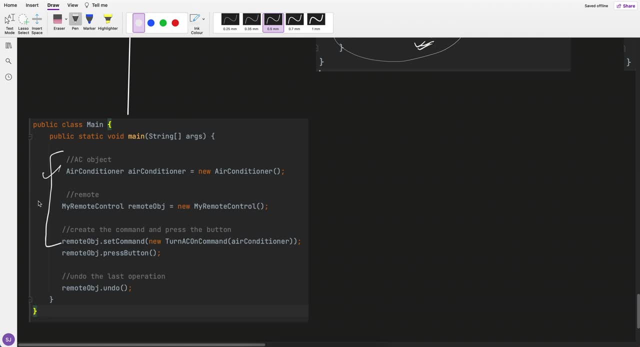 command and you can call that particular command undo operation, okay, and the client simply has to do. this is just a setup. i have set up an ac, i have an hour remote and let's say, in the remote i have set the command to turn on the ac, turn ac on command. right now i am. 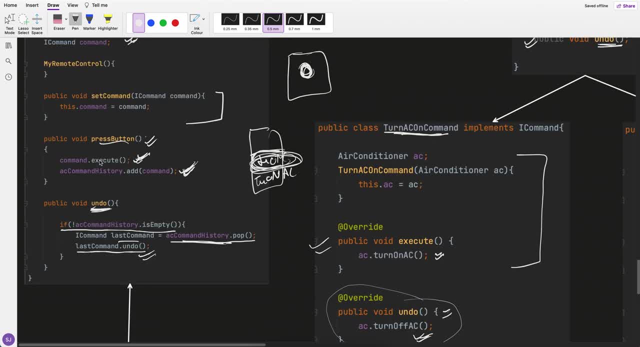 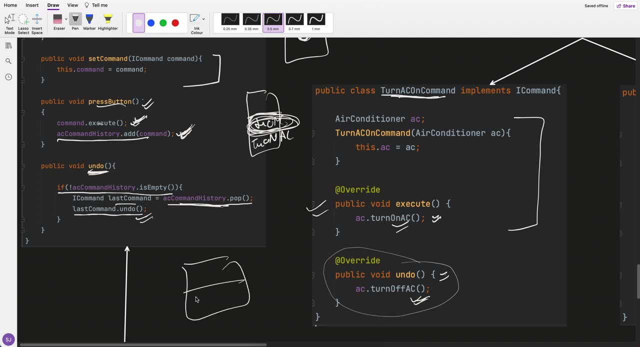 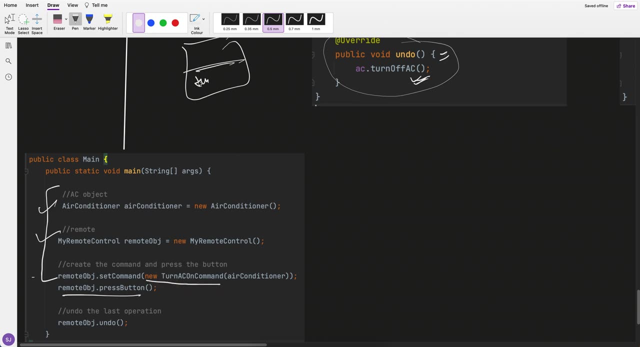 just pressing the button. what it will do is press button. it will command dot, execute, it will turn on the ac and after that it will put into an stack this command. right, this is the command. turn ac on command. it will put into the stack. now i wanted to. 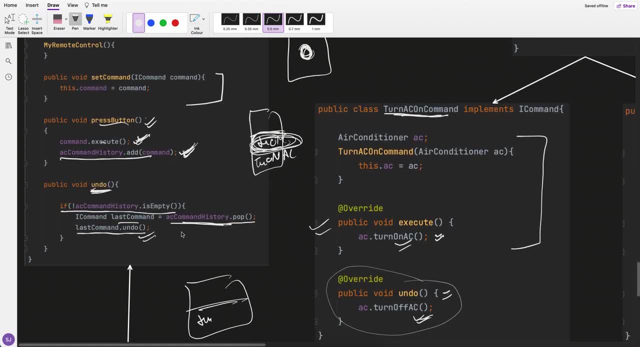 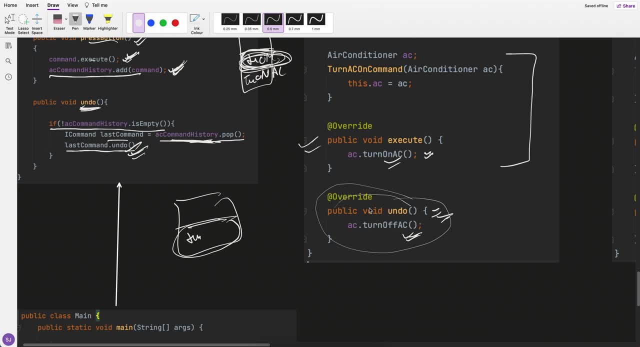 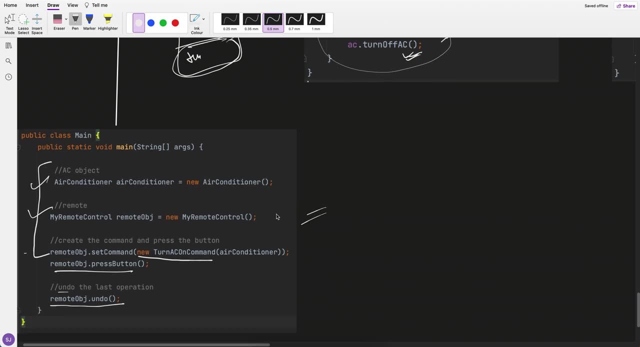 undo. i will just simply call undo method. what it will do is it will take out from the pop: okay, turn ac on command. it will call its undo method. it will revert what it has done. so the client doesn't have to worry about the undo redo functionality, it just has to invoke. 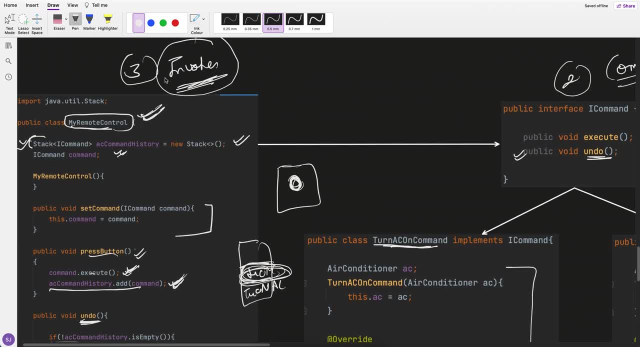 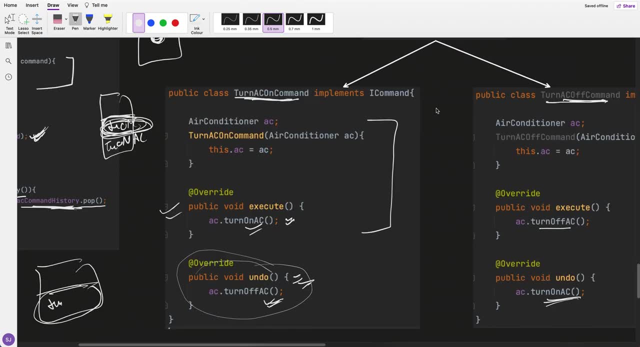 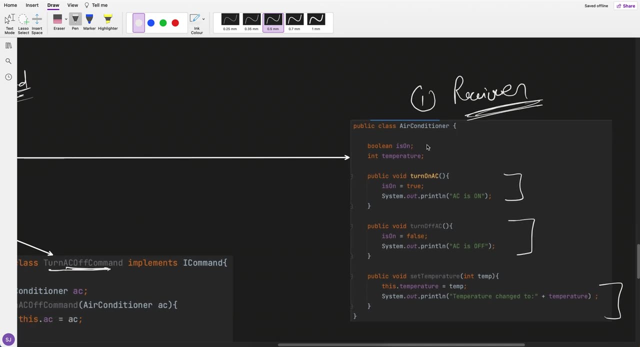 undo. and here it: invoker maintain a list of the commands in a stack right and the functionality of reverting the command operation is taken by the command itself. so here receiver is just dumb object. it only, like it, totally depend upon the command to change its status right.